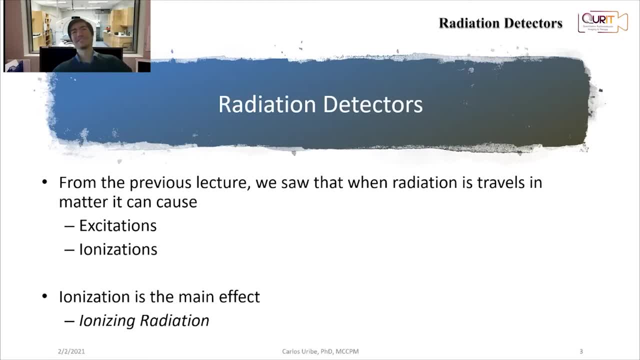 electrons, Because this radiation causes ionizations. that's why an ionization is the main effect. That's why you typically hear the name of ionizing radiation, And ionizing radiation is the one that you typically hear being very bad because these ionizations, for example, can cause well, that's basically. 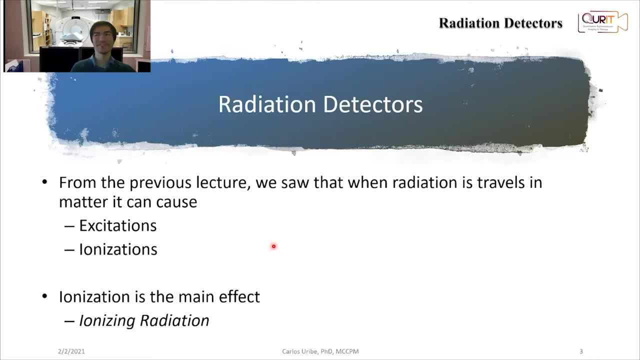 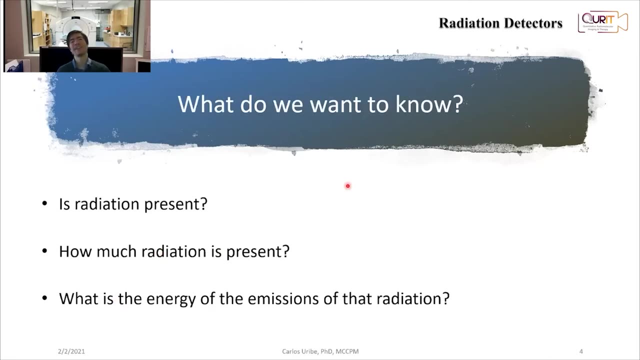 what's causing bad effects on the DNA of cells? because ionizations then make free radicals that they end up combining with different things or damaging the DNA. So it's ionizing radiation- also a name for radiation. So what is it that we want to know when we think of building detectors? So we want to. 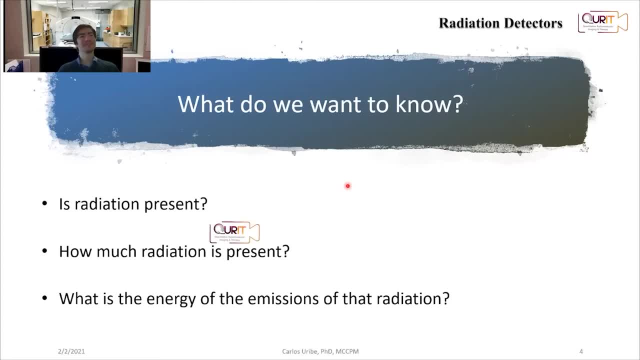 see if maybe what we want to be able to detect radiation, of course. is there radiation present? If there's radiation present, is there a way for us to quantify how much radiation is there? And if we know that there's radiation there, is there any way for me to know what are the 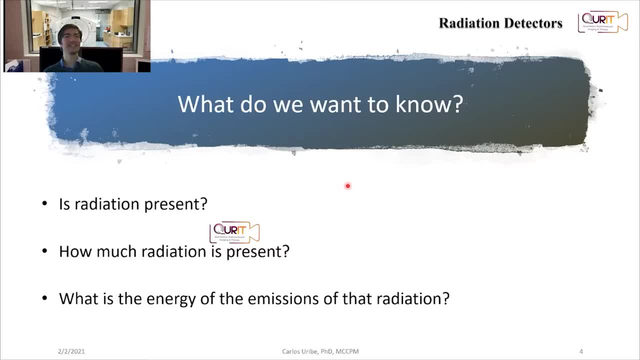 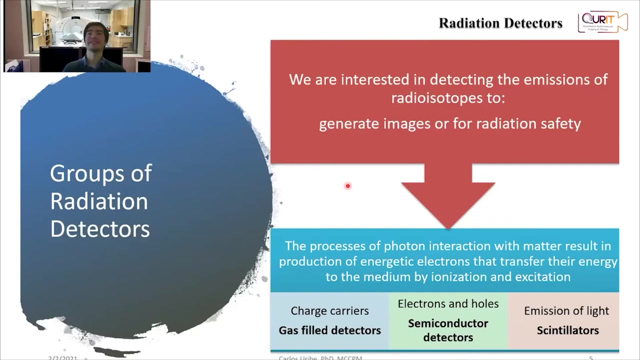 energy of the emissions Coming out of there. Is there a way for me to know, for example, if a particle is a beta particle, or if I'm measuring, or if the radiation that I'm seeing are photons or alpha particles? So we have several groups of radiation detectors and we are interested well for the 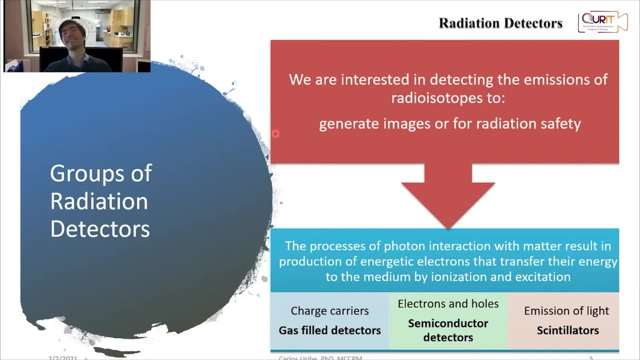 particular case of nuclear medicine. we're interested in using the radiation to generate images, but then we also use detectors in the nuclear medicine, not in the nuclear medicine application itself, but in the nuclear medicine practice in the hospital, For example. we need to be careful with staff exposure to radiation, so we use detectors. 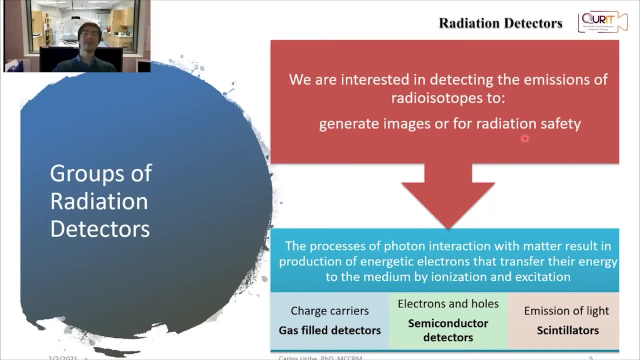 for radiation safety And the processes of photon interaction with matter. Okay, so when we have photon interactions, we just need to keep in mind, remember photons don't directly deposit energy in the medium, It's more like the electric field. But these photons are going to create free electrons in the medium and then these free 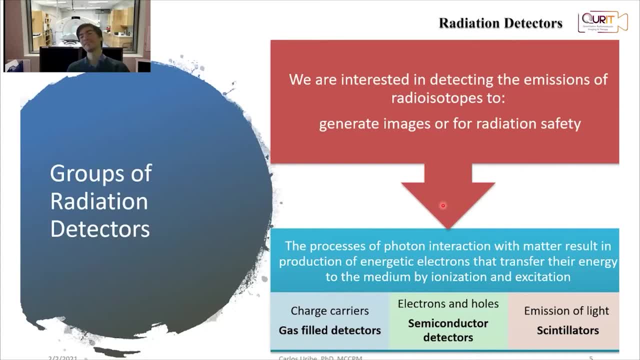 electrons are going to transfer their energy to the medium by that ionization and excitation. We have different types of detectors. We have what we call charge carriers, which typically are gas field detectors. We have semiconductors detectors in which we deal with electrons and holes. 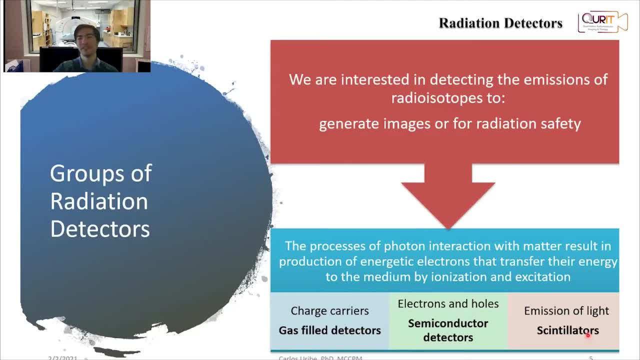 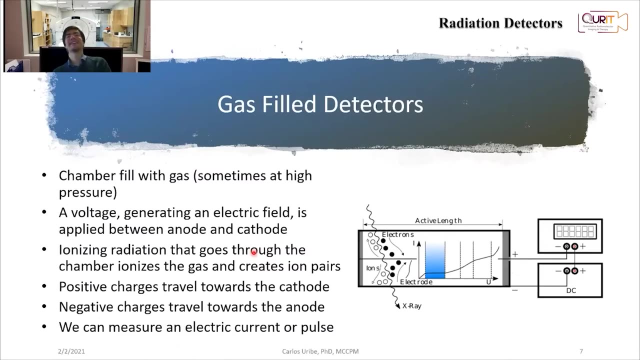 And we have what's called scintillator detectors, which are some detectors that emit light when there's interactions with radiation. Let's start talking about gas field detectors. So what is a gas field detector? You can think about having a chamber that is filled with a gas. 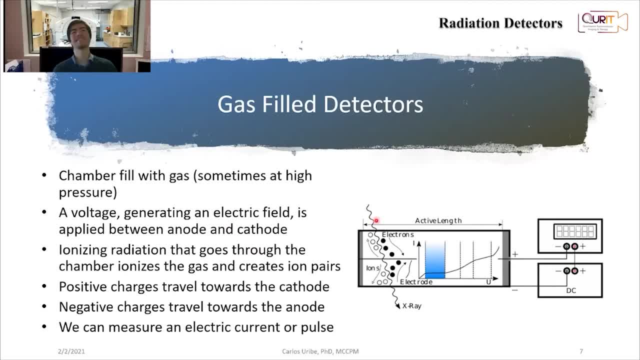 So imagine just a little device that has some gas inside, Now that gas can either be pressurized gas or it can just be basically air. It's just exposed to the air And that gas is going to be charged by the atmospheric pressure. 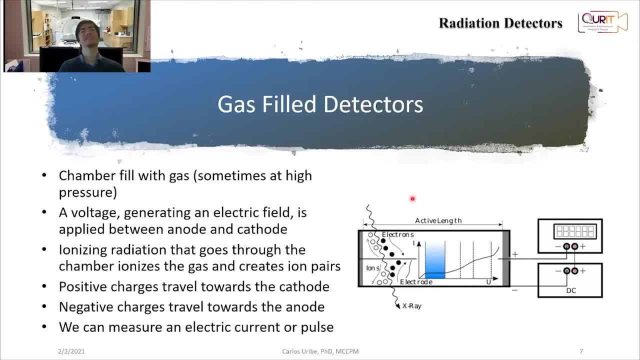 We can put a different voltage between two electrodes. One is what we call the cathode, which is going to be the negatively charged electrode, And we have the anode. Wait, am I saying that right? No, the anode. Yeah, the anode is going to be positively charged and the cathode is going to be negatively. 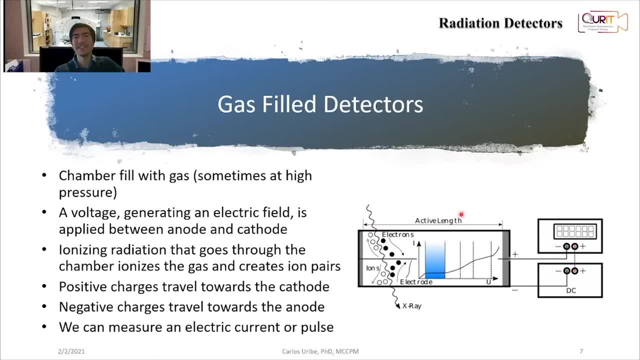 charged, And what you have then, when you put this anode and cathode- one is positive, one is negative- What you have there is that you generate an electric field. So there's this difference in voltage that causes an electric field. 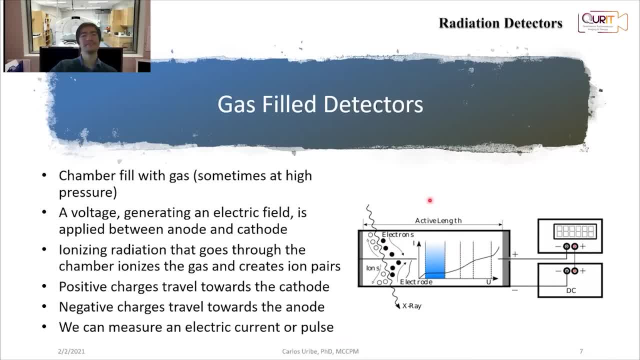 So when ionizing radiation goes through this chamber, well, again because of the name, it causes some ionizations. So in this gas we're going to have some positive and negative ions. So now we have these charges, So positive charges are going to move towards the negative. 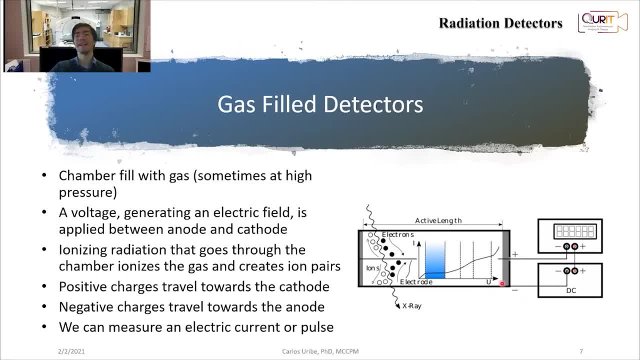 Well, like pole of the battery, And negative charges are going to move to the positive side again because of that electric field there. So positive charges travel to the cathode, which is negative. Negative charges travel to the anode, which is positive. 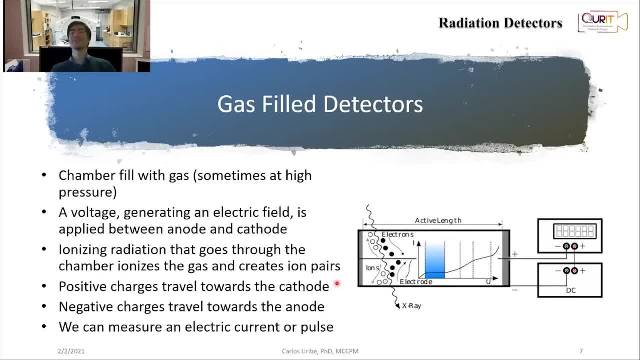 And when we do this, when these charges are moving, what we can measure on the other side of the device is an electric pulse or an electric current. OK, But then let's think about: OK, we can have this anode, this cathode. 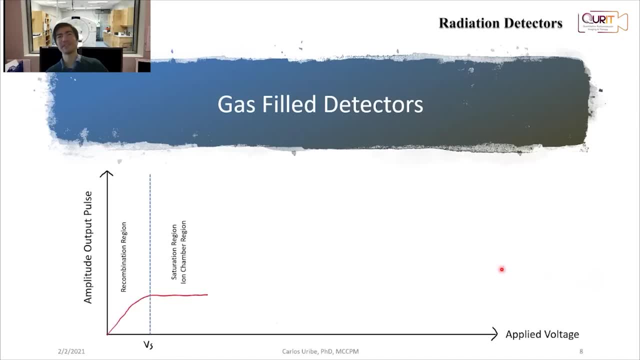 What's the voltage that we can put there So we can start building a graph in which we're going to start increasing the voltage of that ionization chamber, that gas field chamber. So if we start from zero voltage and then we start applying a little bit of a voltage, 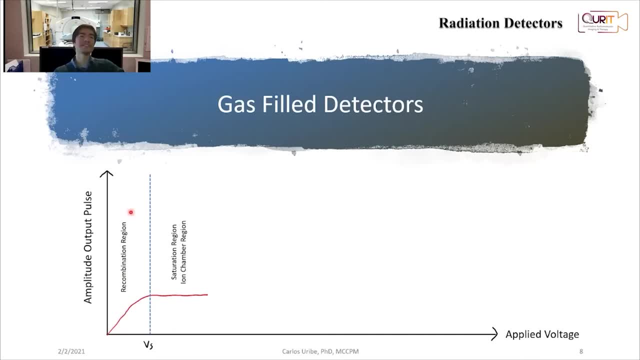 and then start growing and growing. we see first this region that is called the recombination region. So what is a recombination region? is that the particles that are traveling into this gas. They create ionizations, But the electric field is not that high. 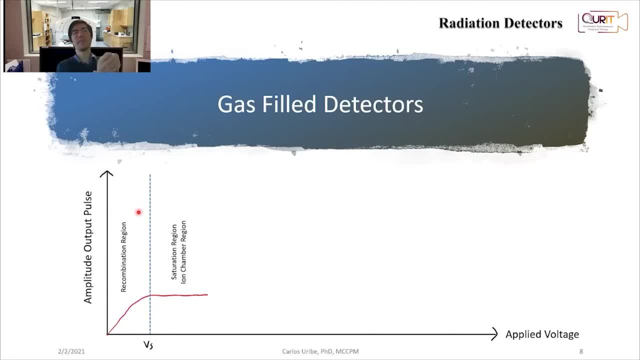 So these ions then recombine by itself before even reaching the anode of the cathode, And yeah, So they become neutral again. And as we start increasing the voltage we get a higher amplitude of the pulse, But some of them at little voltages don't really make it to the other side. 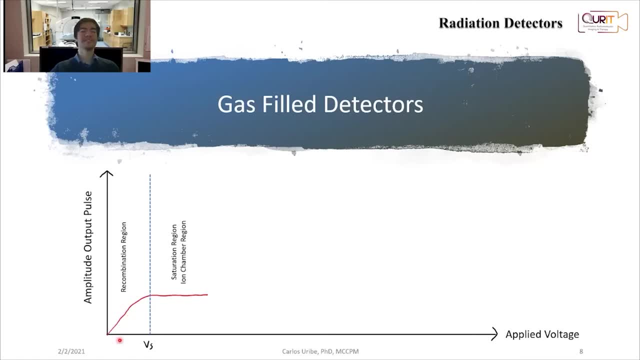 They don't give as much of an output pulse. But as we start growing then it starts increasing, Increasing the pulse. Then we get to a voltage that we call the saturation voltage And this brings us to what we call the saturation region. 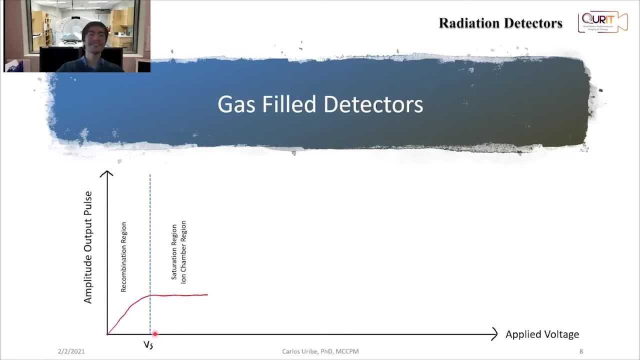 So what this means is, although we keep increasing the voltage, we don't really see too much difference in the collection. We don't really see a difference in the collection of the charge or in the collection of that pulse that we're able to measure. 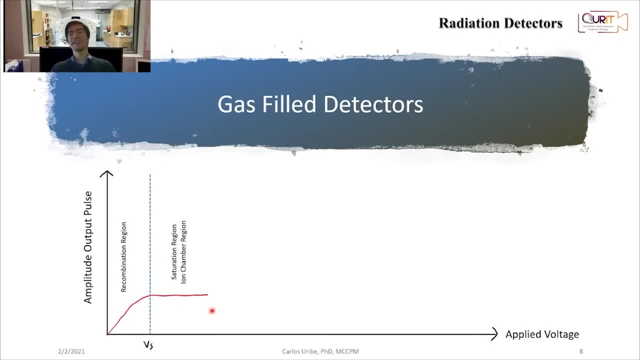 The reason for this is that all the charges created inside the gas By that ionizing radiation is being collected, So we're basically collecting all the charges. No matter if you apply a little bit more voltage, you're still collecting all the charges that. 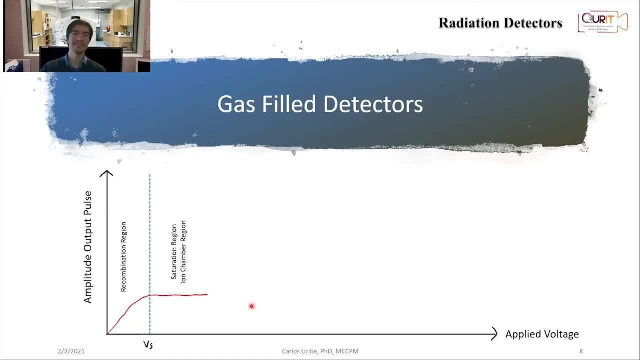 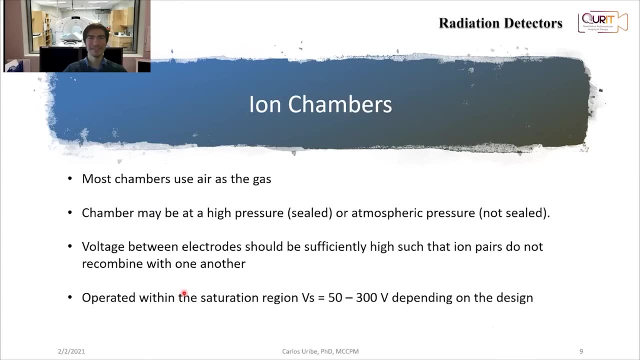 are generated, So that's why that output is not created. And this region, in which we call either the saturation region or the ion chamber region, is what brings me to the first type of detectors, what we call the ion chamber detectors. Now, most of these ion chambers use air as the gas. 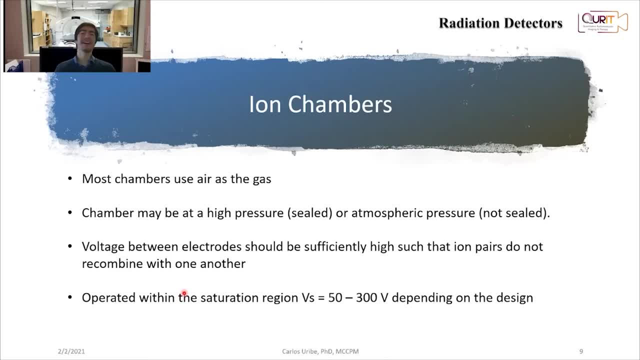 So, as I said before, these chambers may be at a high pressure. So, of course, if you have high pressure, that chamber has to be sealed Or it can be exposed to the atmosphere. So it's not sealed, It's just atmospheric pressure. 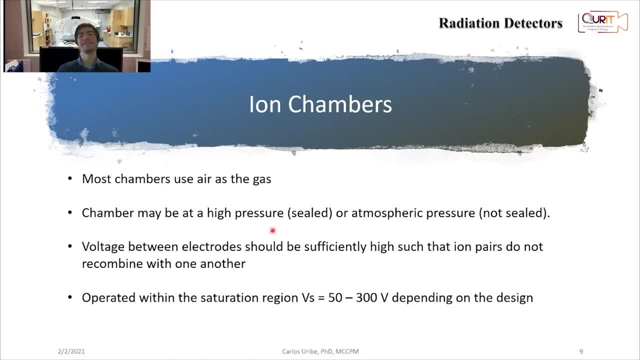 Now the voltage between the electrodes should be high enough that the ion pairs do not recombine with each other. So again that recombination region. we now want to collect all the charges. We don't want some of them recombining itself. 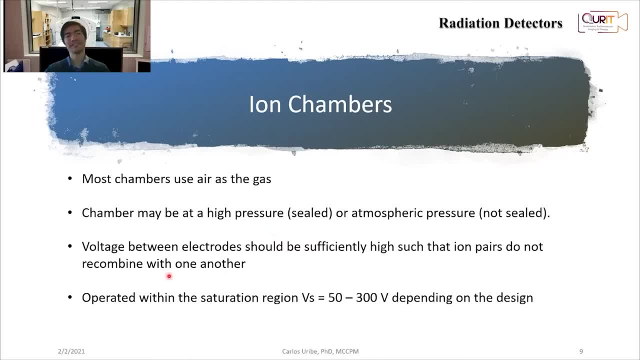 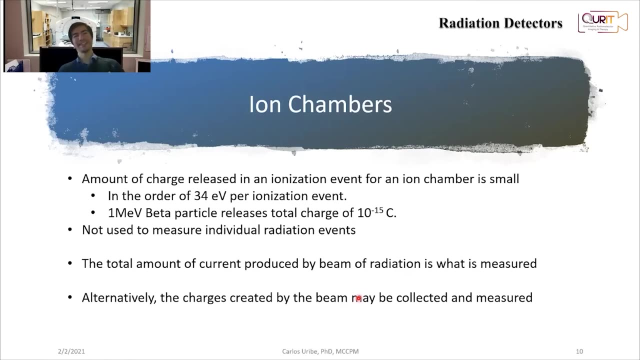 And losing them in the process, So that voltage tends to be sometime in the order between 50 to 300 volts, depending on the particular design of the chamber. While here we're talking about a gas, The typical amount of charge released in an ionization event from an ion chamber is small. 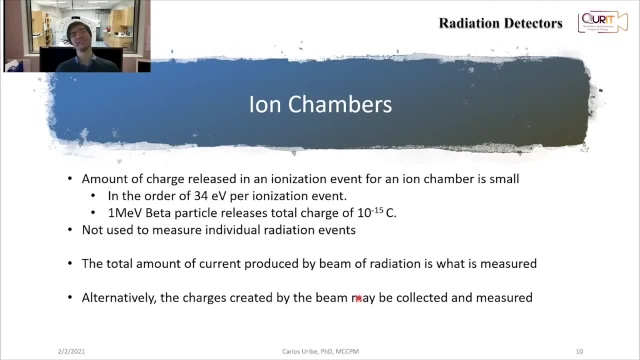 It's in the order of 34 electron volts per ionization event. So basically you need about 34 electrons electron volts to create one ionization event. When you think about a one MeV beta particle, that releases a total charge of approximately 10 to the negative 15 coulombs. So in total, 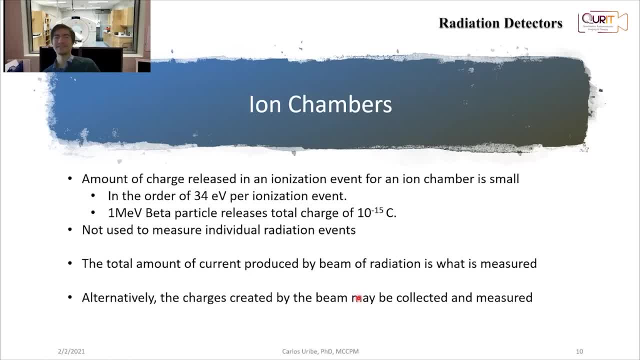 we collect the total, charge, the total- yeah, total- ions of 10 to the minus 15 coulombs. Ion chambers, then, are not really used to measure individual radiation events, because the collection is just very small. So what we measure is just the total current produced by that beam of radiation. 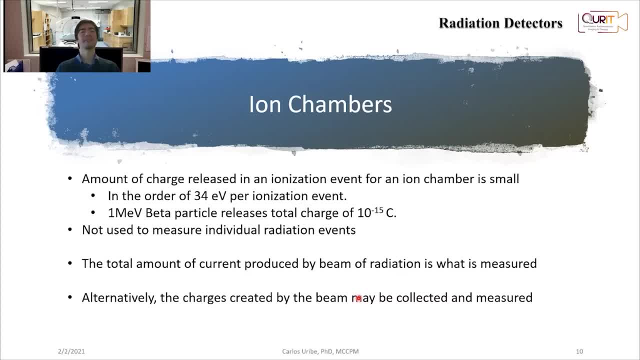 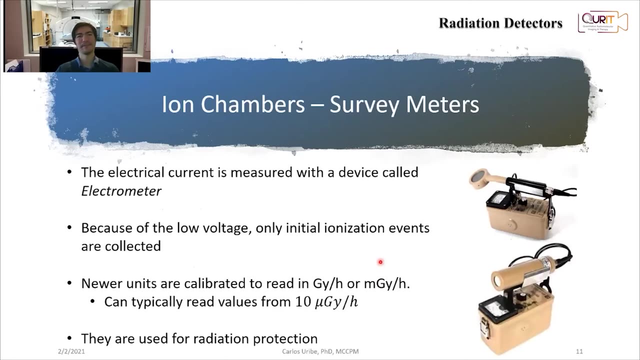 So we see, we just collect the height of the pulse on the other side- not on the other side, but on our measuring device. Yeah, so you can either measure the current or you can see how many charges you collected. Now, ion chambers are typically used in what we call survey meters. 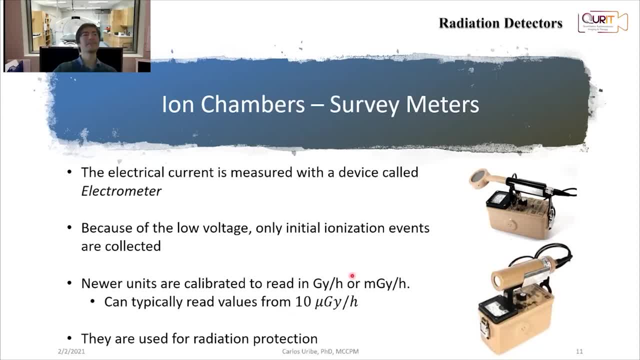 And these are just two photos of how a survey meters can look like. So well to be able to measure that current now, instead of me saying in the other side what's typically being done, we use a device that is called an electrometer. So electrometer, we plug it into our chamber. 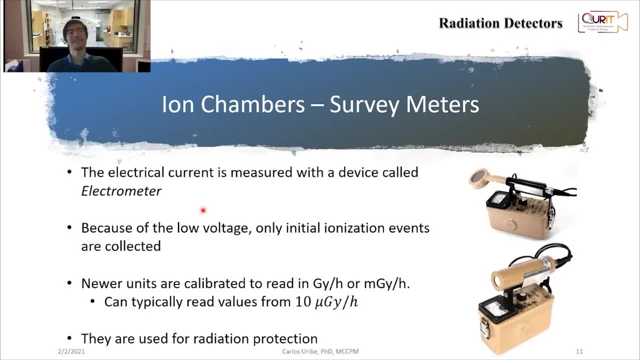 and now we're able to collect, either charge or measure our current Because of the low voltage again I said only at the ionization events caused by that initial- but that radiation that is hitting the chamber is collected, And what I mean with this. 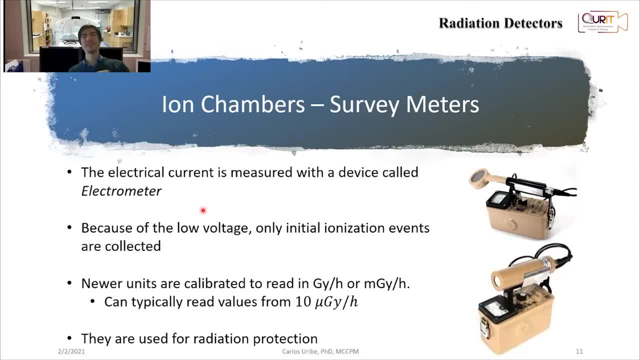 and we're going to say this in a moment- is this voltage will create ions, but those ions are not going to be energetic enough to create more ionizations, So we're only collecting the ions that come directly from the interaction of that radiation with our gas chamber. 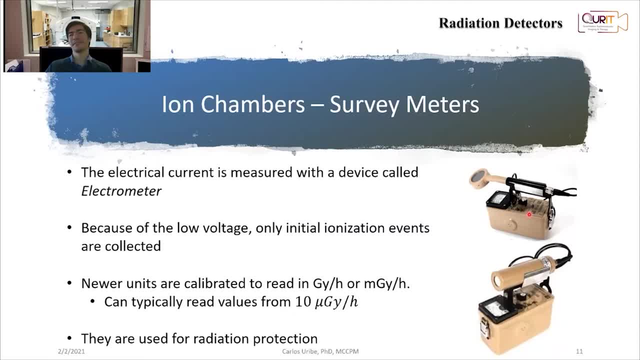 The newer units- oh sorry, yeah so- are typically current equipment. they are calibrated to read values in milli-grade per hour or grade per hour. basically it's a dose rate Again at some point in the course we're going to. 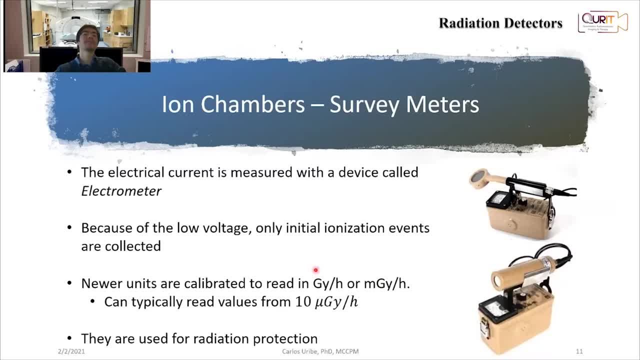 understand much better what dose really means. but this is how much energy per unit mass gets deposited per hour. So we're measuring a dose rate And they can typically read values from 10 micrograde per hour up Now. do we use these devices really to create images of a patient? 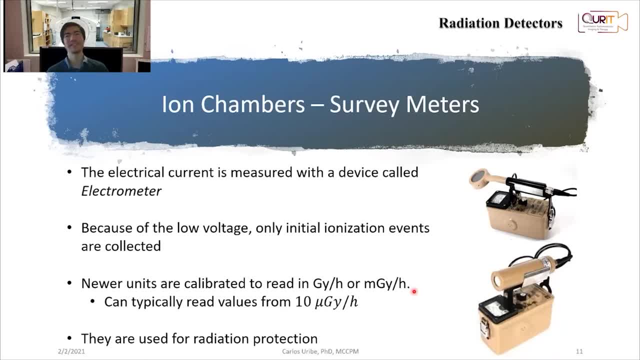 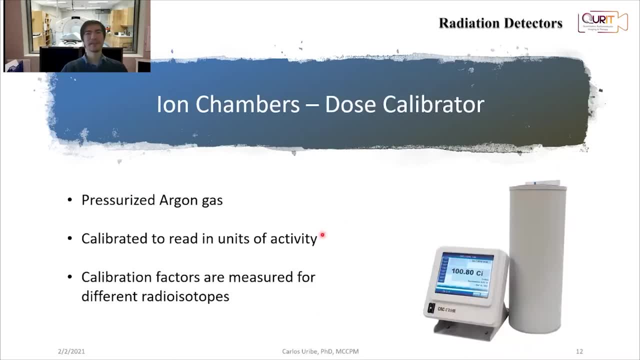 Well, not really. They are just mostly used for radiation protection. If you want to detect if there's some radiation around or if there's some contamination, We have another device. We call this device a dose calibrator, So again it's an ion chamber. Now dose calibrators compared to other. 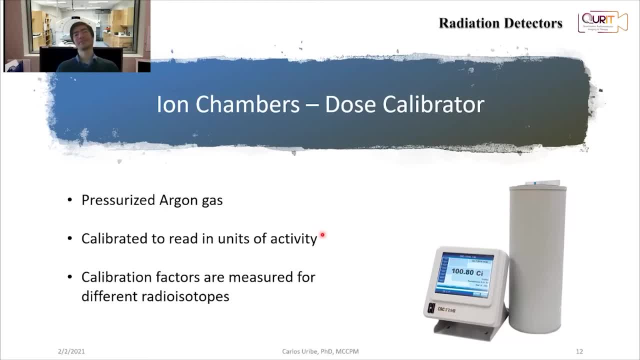 typical gas chambers. they are actually pressurized chambers, So the gas that's containing inside this chamber is typically argon And, yeah, actually one of the reasons that dose calibrators end up failing. they're very robust, but when they end up failing, there's a big chance that. 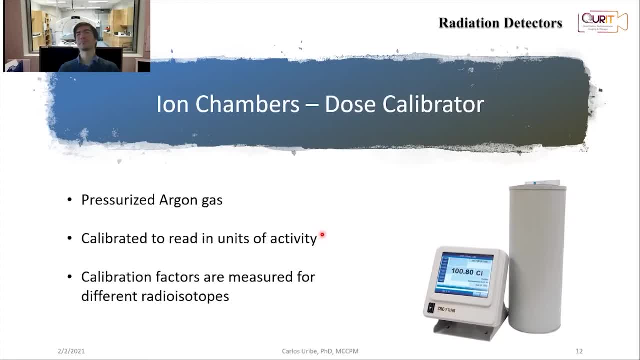 it's because they start leaking this argon gas. So the pressure starts going down and now they're going to start leaking. Now we calibrate this equipment to read units of activity. So what do I mean with that? We actually read mega Becquerel or Millie Curie, for example. But to do this? 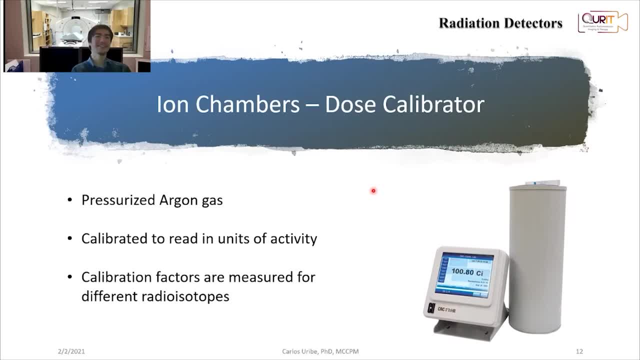 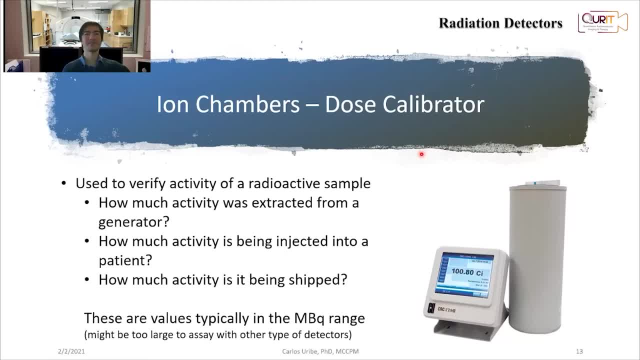 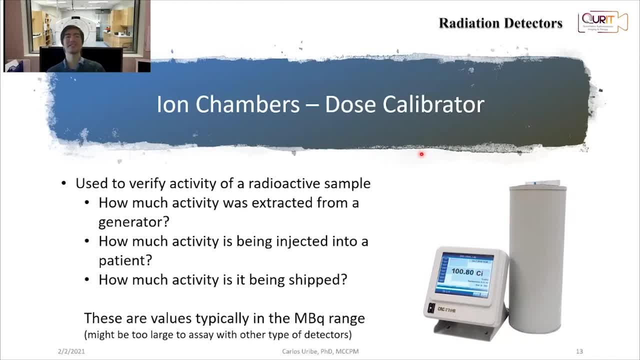 chamber, So we use them to know how much activity comes from the generator. then either we can also activity comes from the generator, then either we can also activity comes from the generator. then either we can also prepare injections and then we see generator. then either we can also prepare injections and then we see. 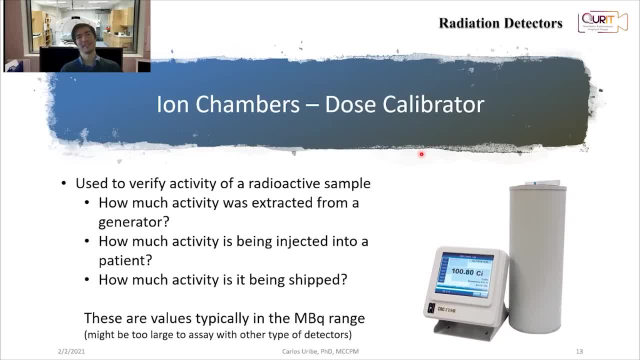 generator, then either we can also prepare injections, and then we see how much activity am I actually prepare injections, and then we see how much activity am I actually prepare injections, and then we see how much activity am I actually injecting into a patient, how much activity am I actually injecting into a patient? Or, if we are dealing with a 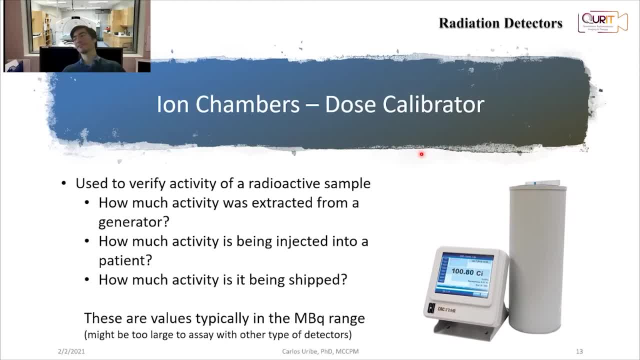 injecting into a patient, Or if we are dealing with a injecting into a patient, Or if we are dealing with a radiopharmacy and the radiopharmacy is, Or if we are dealing with a radiopharmacy and the radiopharmacy is radiopharmacy and the radiopharmacy is preparing samples, then they need to. 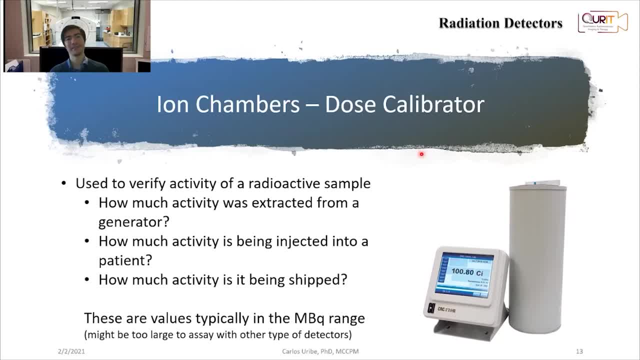 preparing samples, then they need to preparing samples. then they need to ship those samples to different hospitals. ship those samples to different hospitals. ship those samples to different hospitals or different places around the world, or different places around the world, or different places around the world. They need to know how much activity are. 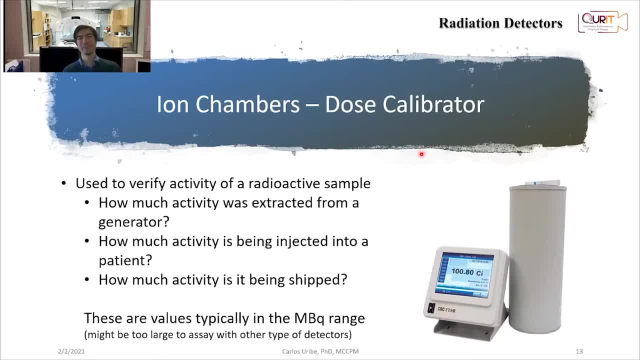 They need to know how much activity are. They need to know how much activity are they shipping. And there's all they shipping. And there's all they shipping. And there's all the regulations for shipments. There's the regulations for shipments. There's. 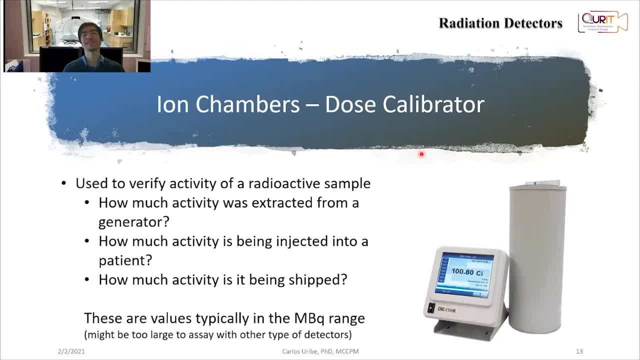 the regulations for shipments. There's, of course, radiation safety involved. of course radiation safety involved. of course, radiation safety involved on what type of injection is safe, on what type of injection is safe, on what type of injection is safe for a patient If you inject too much. 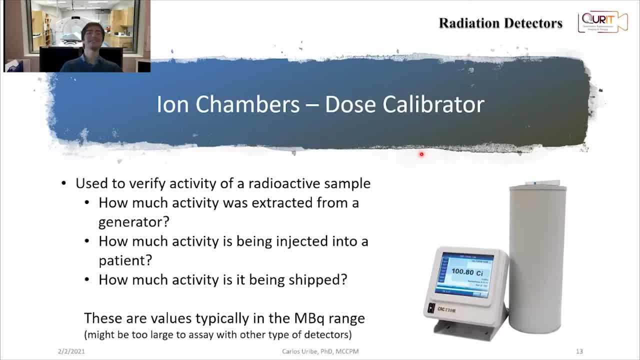 for a patient If you inject too much for a patient. If you inject too much, then you end up getting some radiation. then you end up getting some radiation, then you end up getting some radiation toxicity. If you inject too little, then toxicity. If you inject too little, then 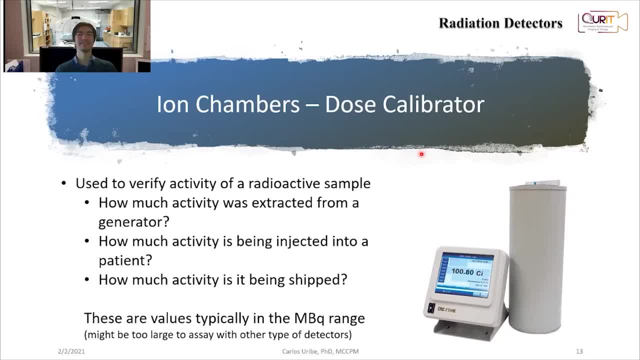 toxicity. If you inject too little, then you maybe won't be able to collect any. you maybe won't be able to collect any. you maybe won't be able to collect any images because there's not going to be images, because there's not going to be. 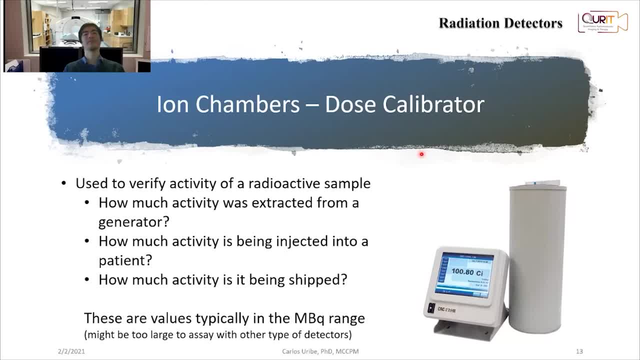 images, because there's not going to be any, any useful information there. So any any useful information there. So any any useful information there. So so this is important Now, these values. so this is important, Now, these values. so this is important Now, these values, the values that we measure in a dose. 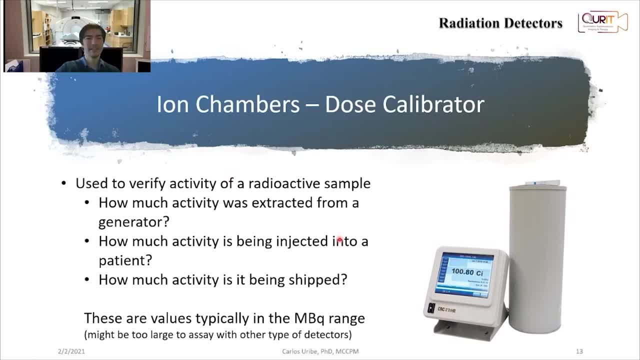 the values that we measure in a dose. the values that we measure in a dose calibrator are typically in the. in the calibrator are typically in the. in the calibrator are typically in the. in the order of the mega becquerel range. order of the mega becquerel range. 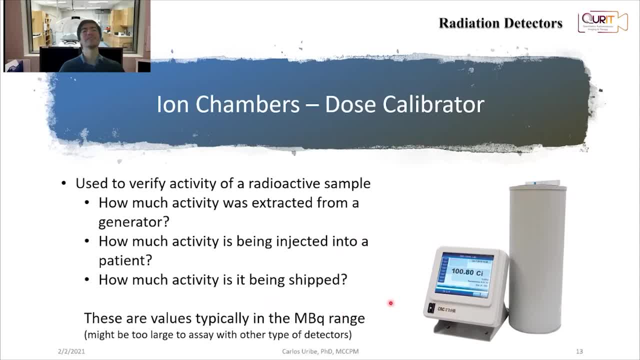 order of the mega becquerel range. because those activity values might be, because those activity values might be, because those activity values might be too large to us with maybe other types too large to us with maybe other types too large to us with maybe other types of detectors like, for example, 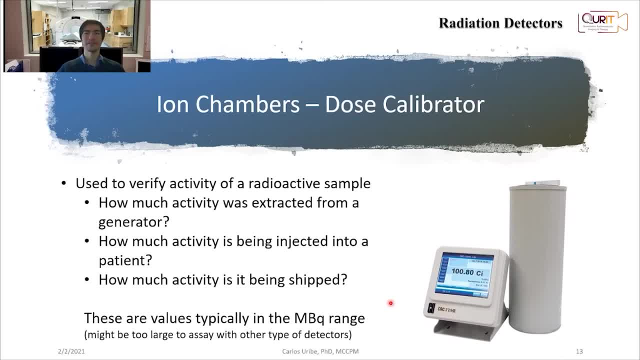 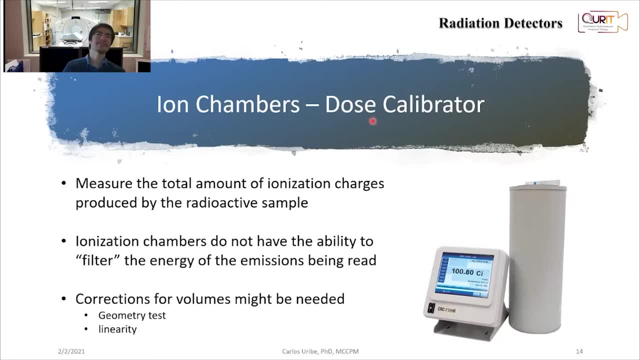 of detectors like, for example, of detectors like, for example, the ion chambers that i started talking, the ion chambers that i started talking, the ion chambers that i started talking about talking with, about talking with, about, talking with, um, um, um. okay, so when we put a sample inside the 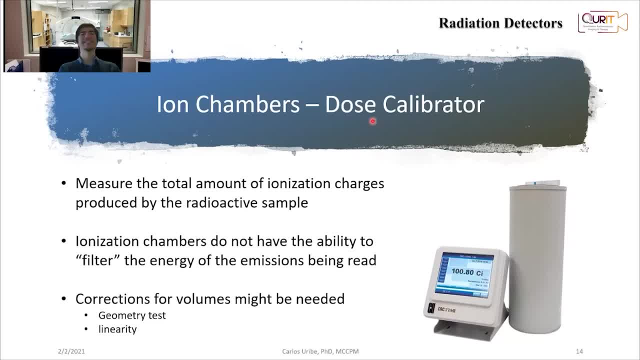 okay. so when we put a sample inside the, okay. so when we put a sample inside the dose calibrator and we're going to look dose calibrator and we're going to look dose calibrator and we're going to look at it a little bit more in detail in the 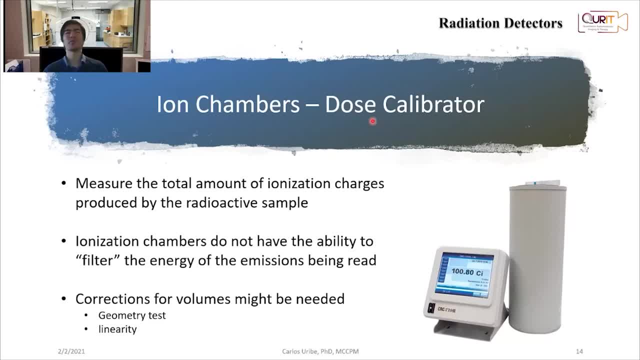 at it a little bit more in detail in the. at it a little bit more in detail in the next lecture, next lecture, next lecture. well, you don't really, you cannot, really well, you don't really, you cannot, really well, you don't really, you cannot really isolate or filter that the energy. 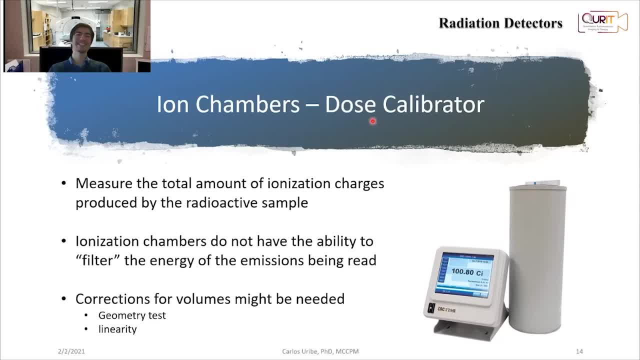 isolate or filter that the energy, isolate or filter that the energy emissions. so emissions, so emissions. so this dose calibrator is going to detect. this dose calibrator is going to detect. this dose calibrator is going to detect all the different particles coming up, all the different particles coming up. 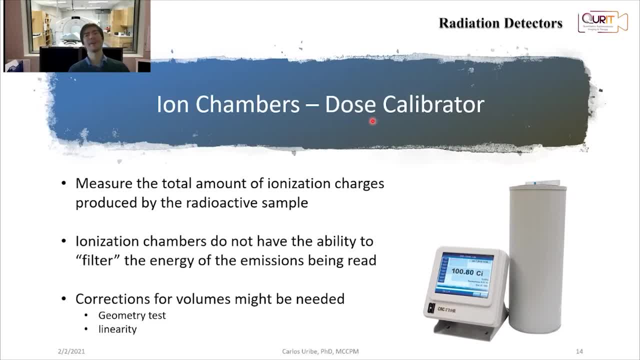 all the different particles coming up from the radioisotope, from the radioisotope, from the radioisotope. so they're going to measure all the. so they're going to measure all the. so they're going to measure all the amounts of ionization charges that this 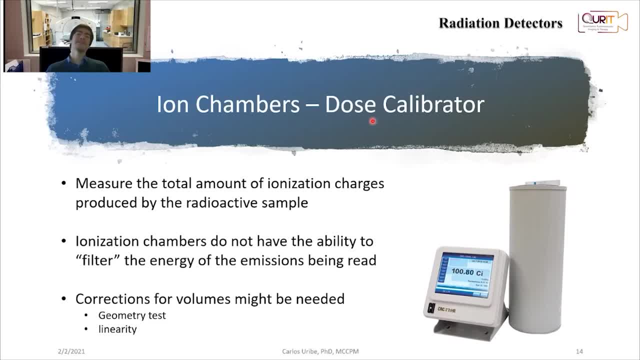 amounts of ionization charges, that this amounts of ionization charges that this sample produces, sample produces, sample produces, and well, and then we need to make some, and well, and then we need to make some, and well, and then we need to make some corrections for it. so what do you think? 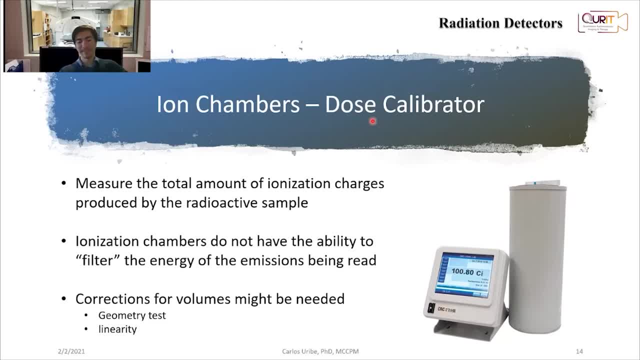 corrections for it. so what do you think? corrections for it. so what do you think? is then? is then? is then. we put a sample in the dose calibrator. we put a sample in the dose calibrator. we put a sample in the dose calibrator. what this sample is doing is it's giving. 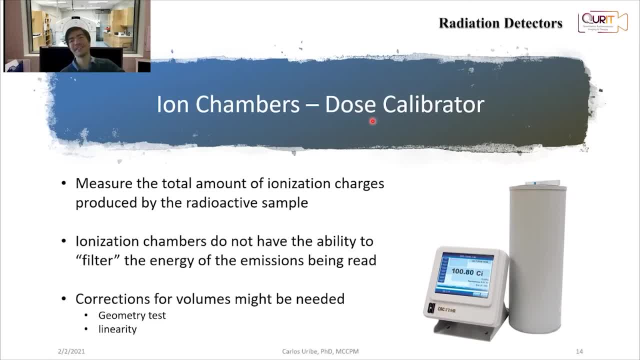 what this sample is doing is it's giving. what this sample is doing is it's giving us, us, us- a current and what we're trying to a current and what we're trying to a current and what we're trying to calibrate is okay. calibrate is okay. 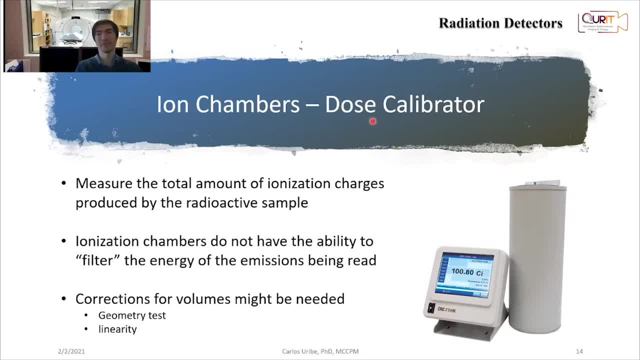 calibrate is okay for this amount of current. how much is for this amount of current? how much is for this amount of current? how much is the activity for this radio isotope? the activity for this radio isotope, the activity for this radio isotope? we have to do this for all the different. 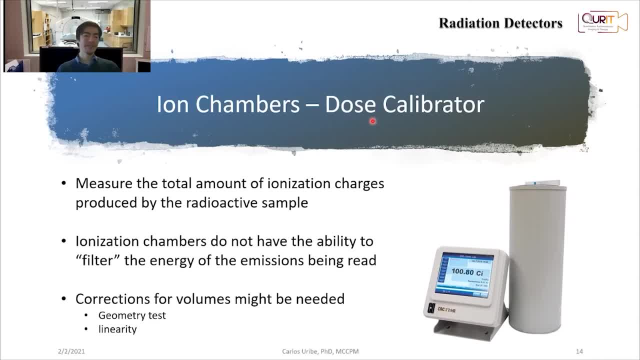 we have to do this for all the different. we have to do this for all the different radio isotopes that are being used in the radio isotopes that are being used in the radio isotopes that are being used in the clinic, because clinic, because clinic, because because things that can happen, because 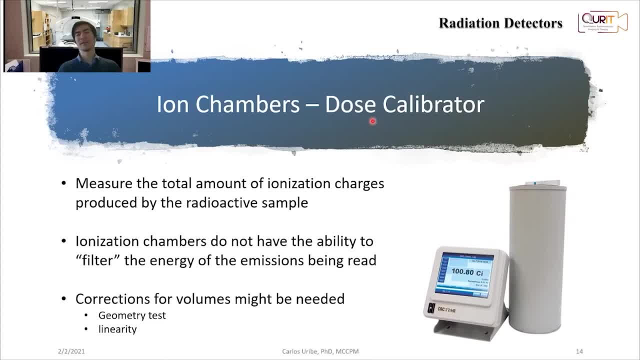 because things that can happen, because, because things that can happen. because isotopes have different emissions and isotopes have different emissions, and isotopes have different emissions and different energies- different energies, different energies. what can happen is that the same amount. what can happen is that the same amount. 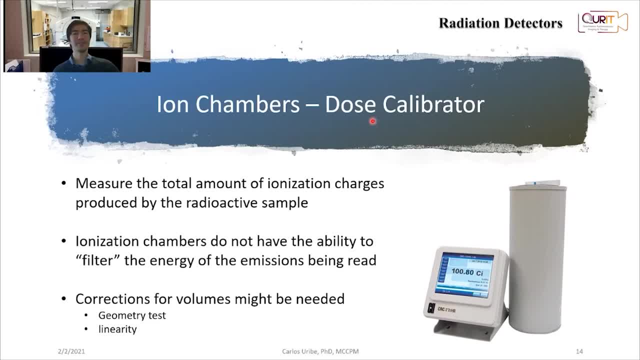 what can happen is that the same amount of activity, of activity, of activity from one isotope, if you have two from one isotope, if you have two from one isotope, if you have two different isotopes with the same amount, different isotopes with the same amount. 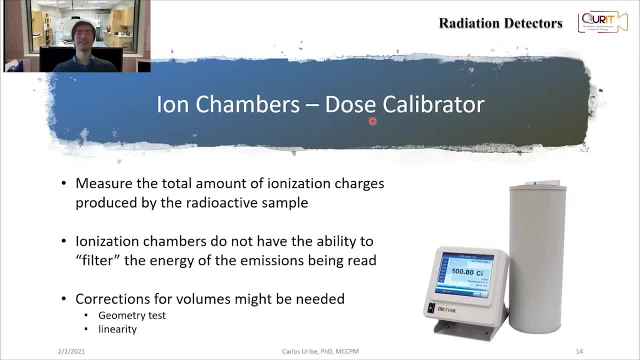 different isotopes with the same amount of activity, of activity, of activity. they can generate different, well, they. they can generate different, well, they. they can generate different, well, they can give you a different pulse current can give you a different pulse current can give you a different pulse current in the ring because, again, the different 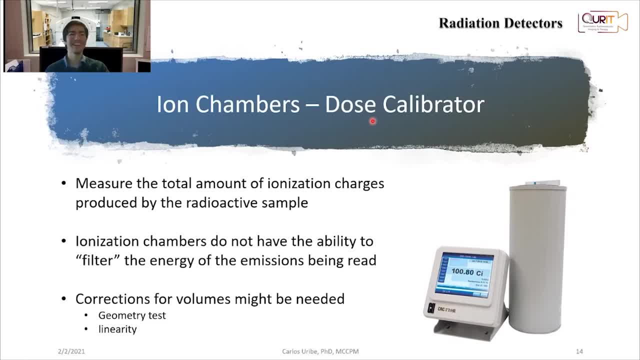 in the ring because, again, the different in the ring, because, again, the different. emission. that is so, that's what we need. emission, that is so. that's what we need. emission, that is so. that's what we need to to to put a known activity a standard. put a known activity a standard. 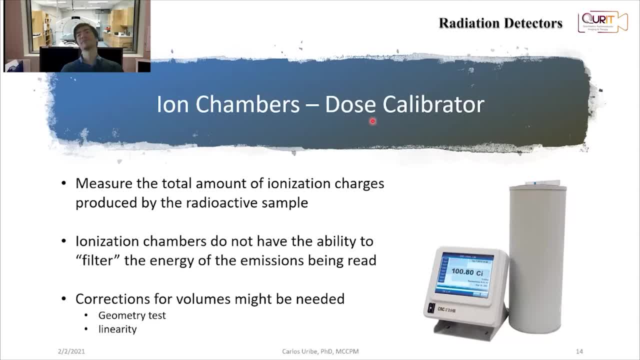 put a known activity, a standard activity, a standardized activity of a activity, a standardized activity of a activity, a standardized activity of a particular isotope, particular isotope, particular isotope, and we have to do what it's called a and we have to do what it's called a. 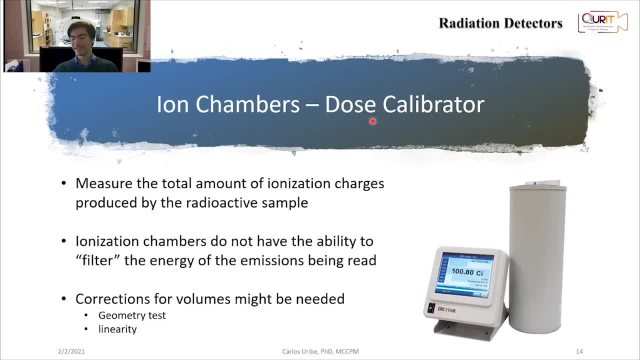 and we have to do what it's called a calibration curve, calibration curve, calibration curve of. okay, these are this amount of of okay. these are this amount of of okay, these are this amount of current for this isotope in particular, current for this isotope in particular. 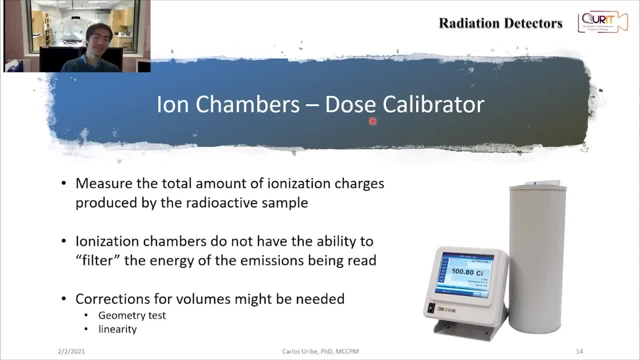 current for this isotope in particular, represents this activity value now for. represents this activity value now for. represents this activity value now for this other isotope, this other isotope, this other isotope. this amount of current represents this, this amount of current represents this, this amount of current represents this activity, and so on and so on, and we do. 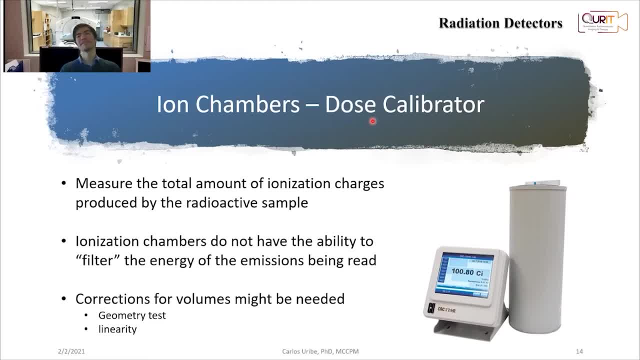 activity and so on and so on, and we do activity and so on, and so on, and we do, we do this for, we do this, for we do this for for many, many different isotopes, and then for many, many different isotopes, and then for many, many different isotopes, and then, if you don't have the isotope, there's a. 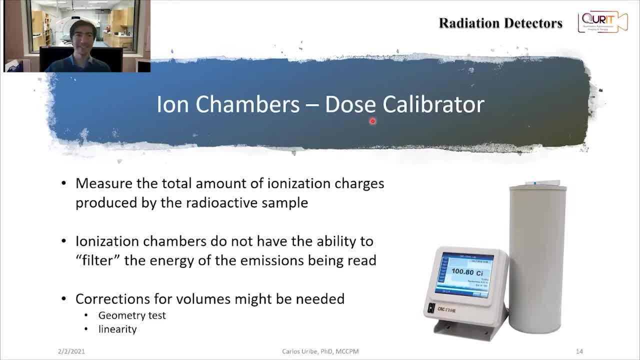 if you don't have the isotope, there's a. if you don't have the isotope, there's a way of interpolating the curve, but way of interpolating the curve, but way of interpolating the curve, but we're not going to get. we're not going to get. 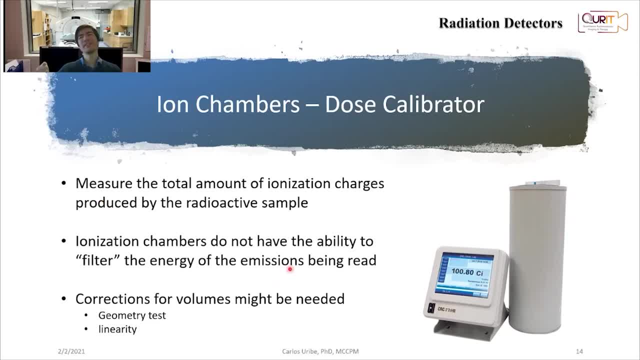 we're not going to get to those details right now, to those details right now, to those details right now. no, nothing you can think is well because no, nothing you can think is well because no, nothing you can think is well because of the geometry of this chamber. 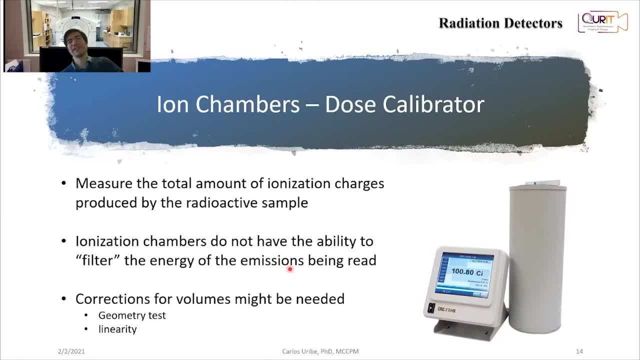 of the geometry of this chamber, of the geometry of this chamber, um, they, um, they, um, they. well, we, we can think that if we put too well we, we can think that if we put too well we, we can think that if we put too much volume or too little volume, it. 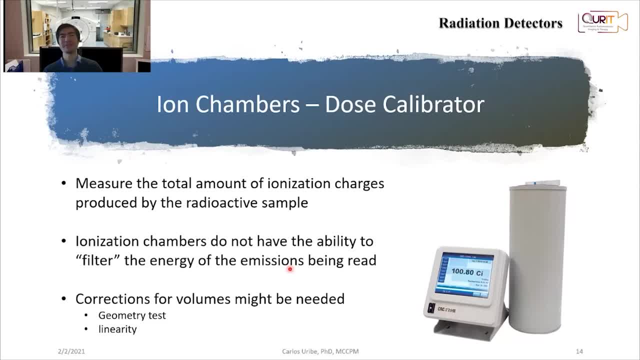 much volume or too little volume? it much volume or too little volume? it might affect the number of ionizations, might affect the number of ionizations, might affect the number of ionizations that you get for a same amount of that you get for a same amount of. 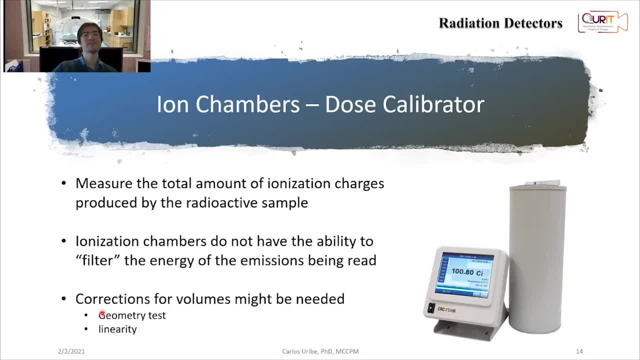 that you get for a same amount of activity, activity, activity. so we do several corrections. we correct, so we do several corrections. we correct, so we do several corrections. we correct volumes by doing what we call the volumes, by doing what we call the volumes, by doing what we call the geometry test. 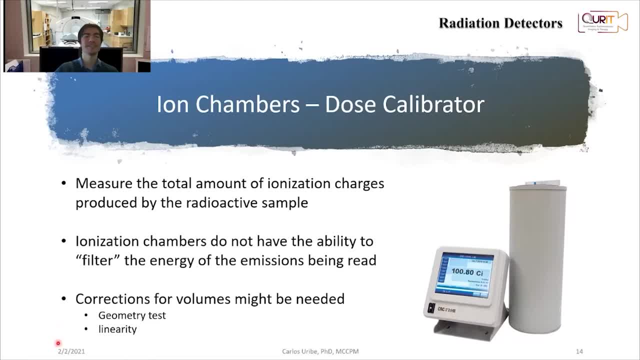 geometry test. geometry test and the linearity: this should be a, and the linearity: this should be a, and the linearity: this should be a. another bullet out here, but another bullet out here, but another bullet out here. but- and we also need to know that, because of 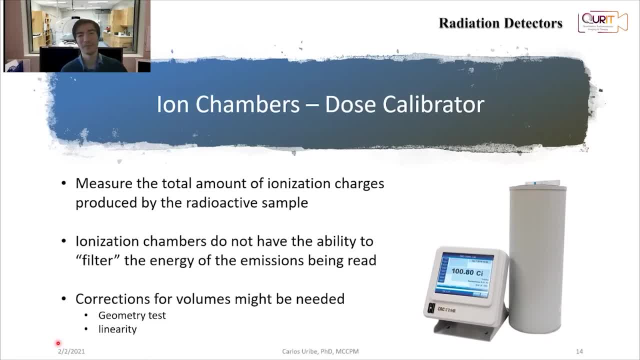 and we also need to know that because of- and we also need to know that because of the way that we're converting, the way that we're converting, the way that we're converting current to activity, but we're making it current to activity, but we're making it. 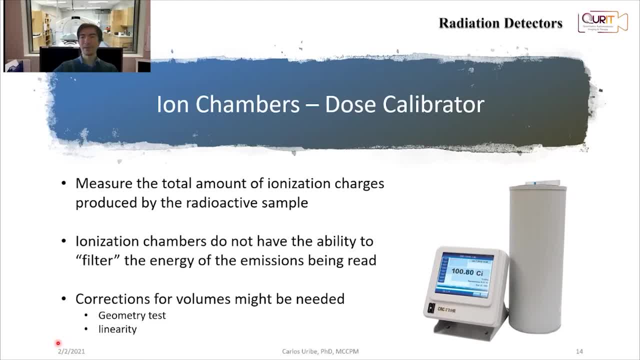 current to activity. but we're making it linear. basically we're saying okay linear. basically we're saying okay linear. basically we're saying okay, i have this current, i multiply by this, i have this current, i multiply by this, i have this current, i multiply by this factor. it gives me some activity. 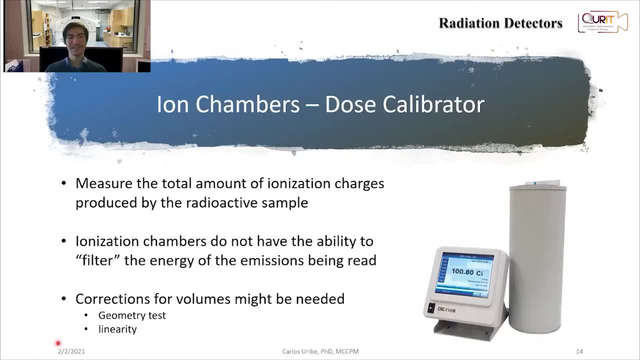 factor. it gives me some activity factor. it gives me some activity. but is that activity? is that factor? but is that activity? is that factor? but is that activity? is that factor going to be the same? if you're going to be the same? if you're going to be the same if you're measuring one mega becquerel, or if 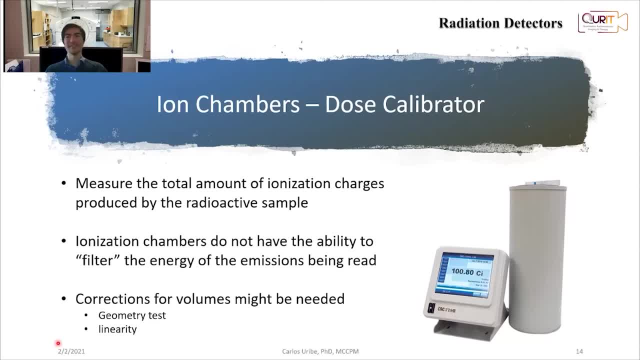 measuring one mega becquerel, or if measuring one mega becquerel, or if you're measuring, you're measuring. you're measuring 100 giga becquerel, for example. if it's 100 giga becquerel, for example, if it's. 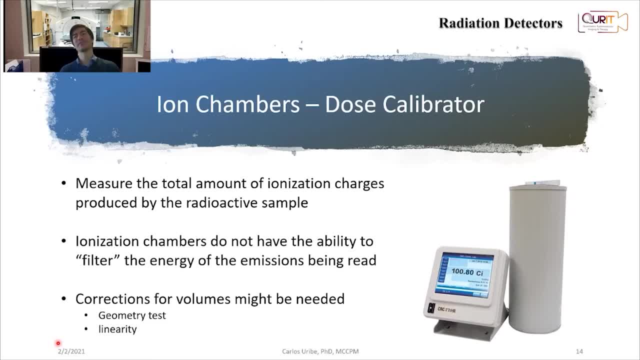 100 giga becquerel, for example? if it's, it's going to be the same calibration. it's going to be the same calibration. it's going to be the same calibration. factor, factor, factor through a big range of different, through a big range of different. 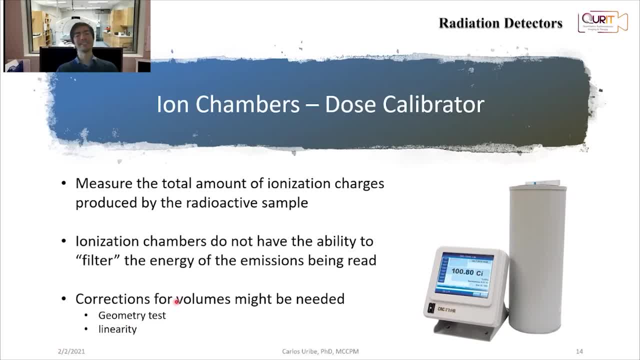 through a big range of different activities. so that's what we call a activities. so that's what we call a activities, so that's what we call a linearity test, linearity test, linearity test, and these are some examples of things. and these are some examples of things. 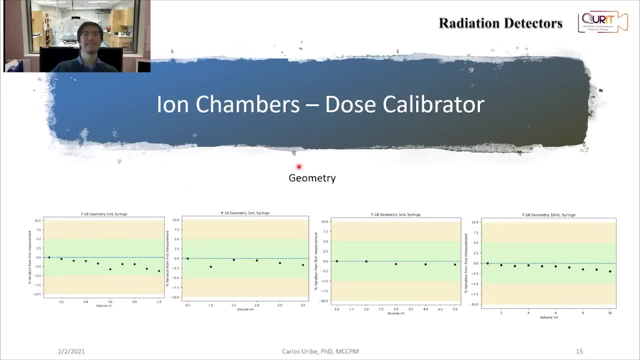 and these are some examples of things that i've done, for example, in our. that i've done, for example, in our. that i've done, for example, in our clinic, clinic, clinic. this is how a geometry test typically. this is how a geometry test typically. this is how a geometry test typically looks. so 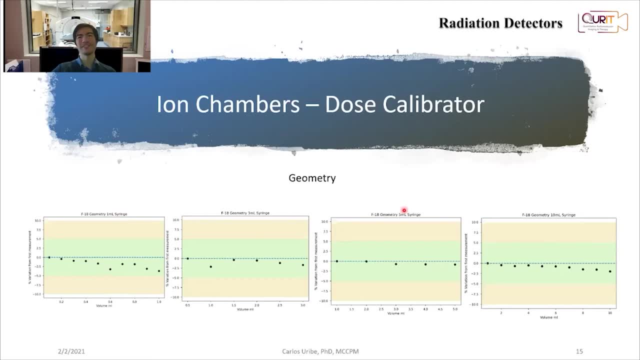 looks so looks. so we perform geometry tests for different. we perform geometry tests for different. we perform geometry tests for different: size of syringes. size of syringes, size of syringes. so again we go from one milliliter. so again we go from one milliliter. so again, we go from one milliliter syringes all the way to 10 million syringes, all the way to 10 million syringes, all the way to 10 million syringes. those are the syringes, those are the. 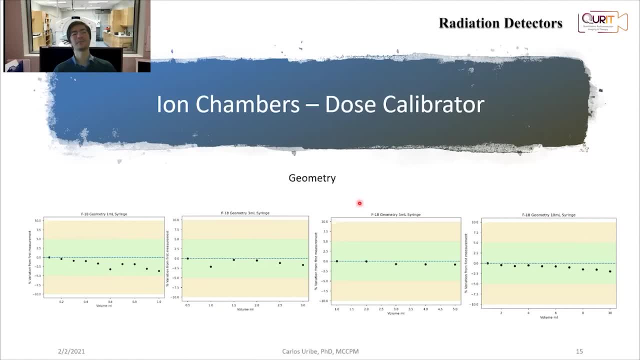 syringes. those are the ones that we typically all. the range is ones that we typically all. the range is ones that we typically all. the range is what we typically use when we inject, what we typically use when we inject, what we typically use when we inject patients. 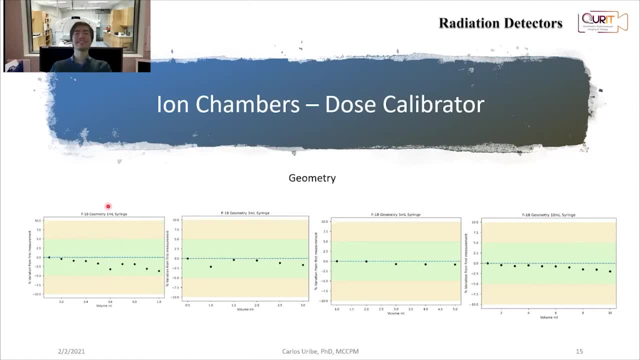 patients, patients. so we just need to make sure that, as so, we just need to make sure that. as so, we just need to make sure that, as we start increasing the volume, we start increasing the volume, we start increasing the volume- our activities are accurately measured. our activities are accurately measured. 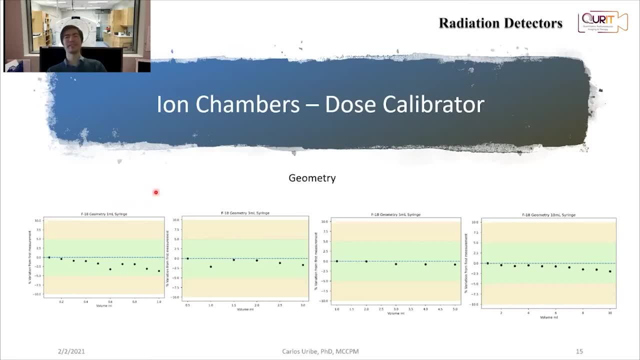 our activities are accurately measured. and one way of doing that is that first. and one way of doing that is that first, and one way of doing that is that first you put a little bit of activity in the, you put a little bit of activity in the, you put a little bit of activity in the syringe and you measure it, and then syringe and you measure it, and then syringe, and you measure it, and then, instead of putting more activity, you put. instead of putting more activity, you put. instead of putting more activity, you put a little bit of saline or a little bit. a little bit of saline or a little bit. 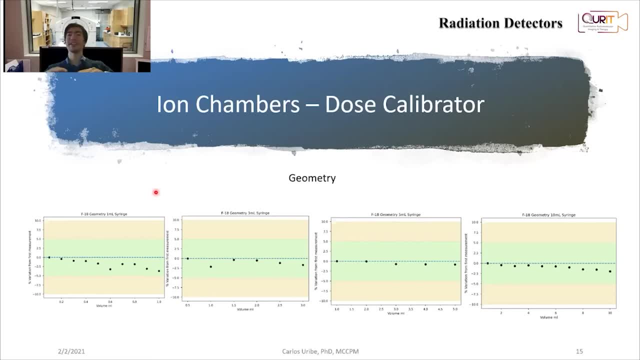 a little bit of saline or a little bit of water, and you measure it again, and of water, and you measure it again, and of water, and you measure it again, and then you put more water, so the activity, then you put more water, so the activity, then you put more water, so the activity is supposed to be constant throughout. 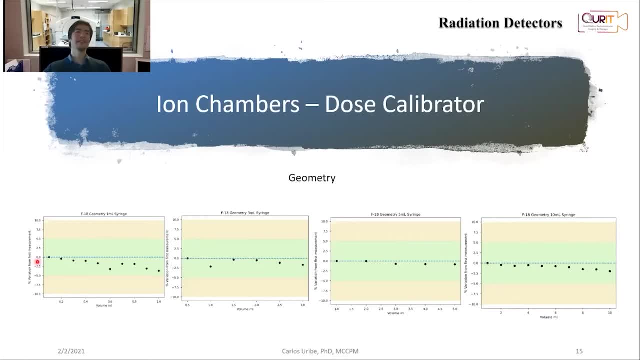 is supposed to be constant throughout, is supposed to be constant throughout your measurement, but you are increasing your measurement. but you are increasing your measurement, but you are increasing the volume, the volume, the volume, and we look to be within five percent, and we look to be within five percent. 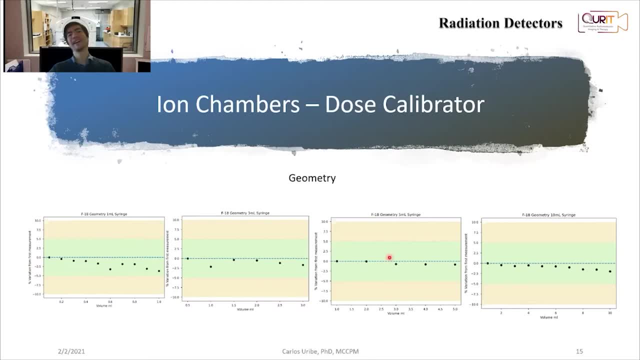 and we look to be within five percent all the time of the initial values, all the time of the initial values, all the time of the initial values. and we do that process for different and we do that process for different and we do that process for different, different syringes. 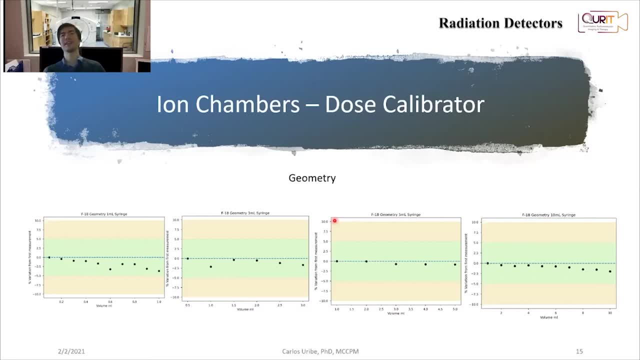 different syringes, different syringes and we. it's a way of checking our and we. it's a way of checking our and we. it's a way of checking our quality of our dose caliber. we just make. quality of our dose caliber, we just make. 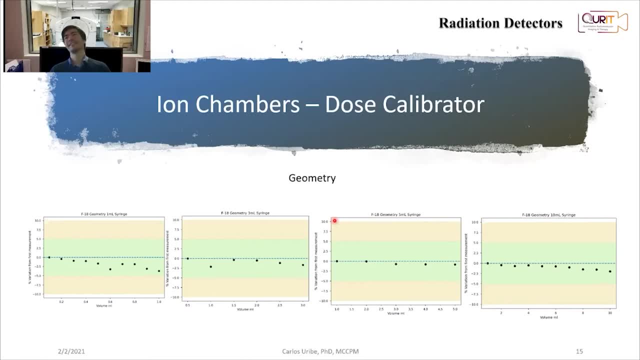 quality of our dose caliber. we just make sure, sure, sure now. if you see differences, then it now. if you see differences, then it now. if you see differences, then it doesn't mean that your dose caliber is doesn't mean that your dose caliber is, doesn't mean that your dose caliber is bad. it just means that you need to. 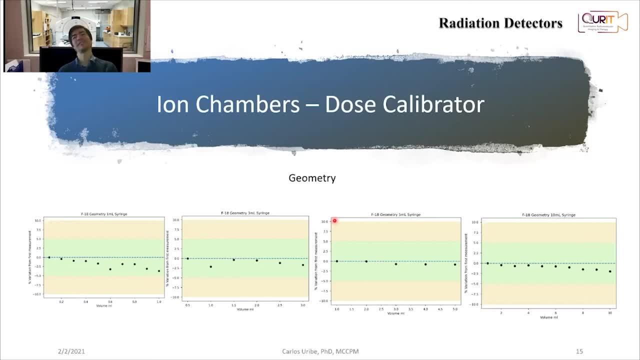 bad. it just means that you need to bad. it just means that you need to account and create another correction account and create another correction account and create another correction factor for different types of geometries, factor for different types of geometries, factor for different types of geometries that you use, so that you know. 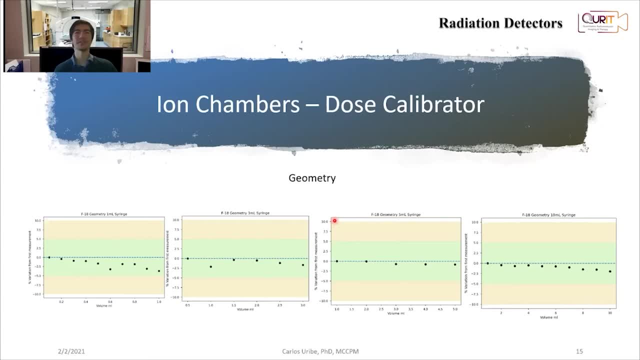 that you use, so that you know that you use, so that you know: okay, if i use this geometry, i know that. okay, if i use this geometry, i know that. okay, if i use this geometry, i know that the reading doesn't correspond exactly. the reading doesn't correspond exactly. 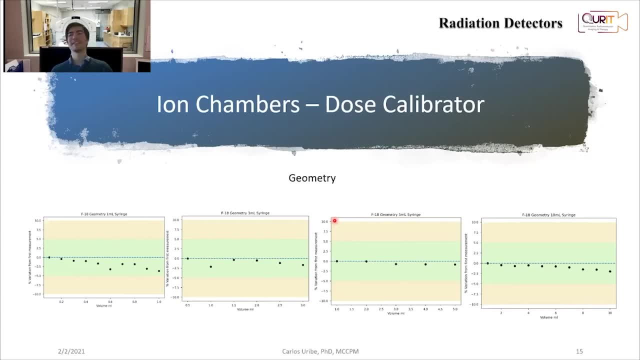 the reading doesn't correspond exactly to what i'm supposed to be having. i need to what i'm supposed to be having. i need to what i'm supposed to be having. i need to multiply my reading. to multiply my reading. to multiply my reading. for for another. 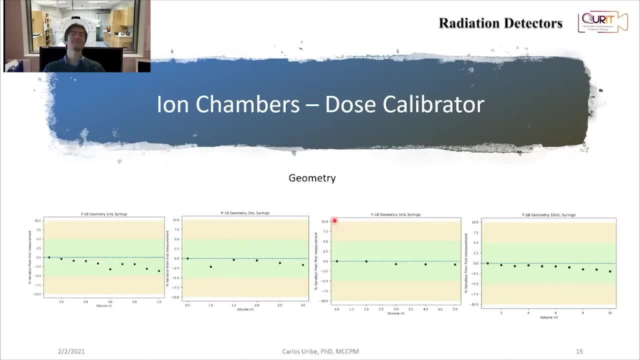 do another correction to, for another correction to, to: to finally get my true value, to. to finally get my true value to, to finally get my true value. and then linearity is what i was saying, and then linearity is what i was saying, and then linearity is what i was saying because of this conversion throughout a 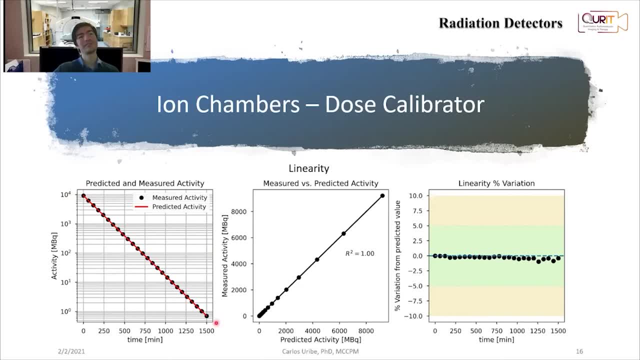 because of this conversion throughout a, because of this conversion throughout a big range of activities. we just need to big range of activities. we just need to big range of activities. we just need to ensure that that's the case, ensure that that's the case, ensure that that's the case. so one of the ways we do this is we, we 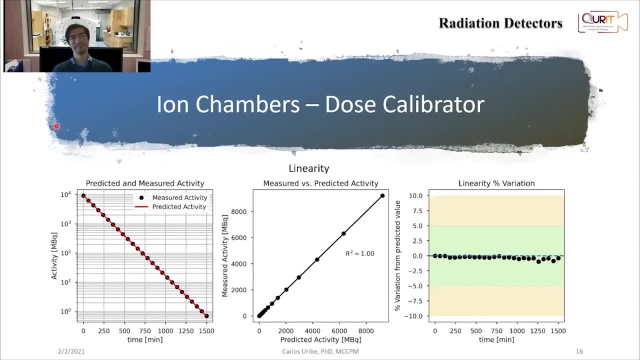 so one of the ways we do this is we, we. so one of the ways we do this is we, we take, take, take a sample of a, a sample of a, a sample of a. well, a high activity, well, a high activity, well, a high activity, and we leave in the dose calibrator. 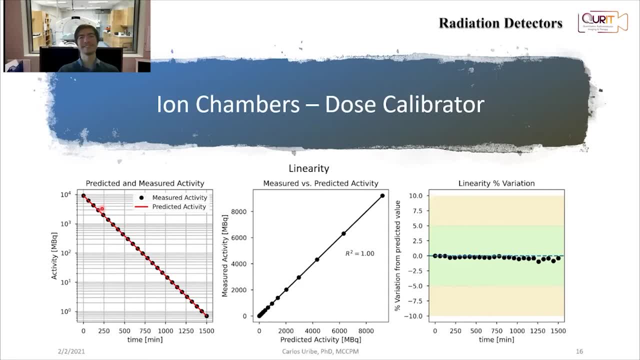 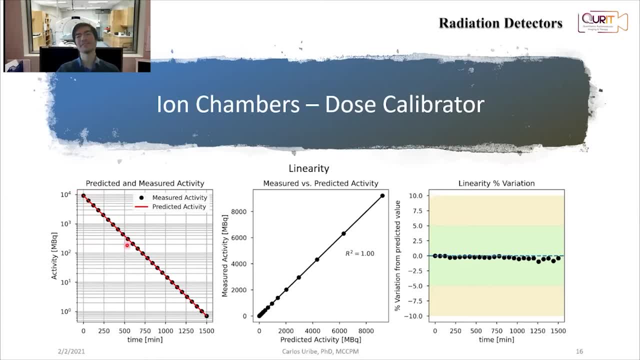 at different times throughout its decay. and well in principle that decay should, and well in principle that decay should, and well in principle that decay should follow. should follow the decay that you follow. should follow the decay that you follow. should follow the decay that you expect, expect, expect. so we know the half-lives of the. 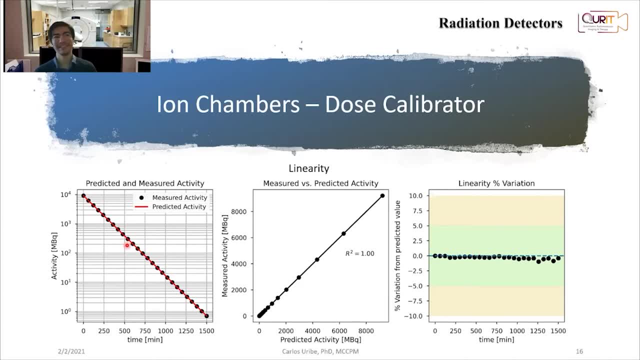 so we know the half-lives of the, so we know the half-lives of the different isotopes. so different isotopes, so different isotopes. so is this actually following that? is this actually following that? is this actually following that half-life and half-life, and? 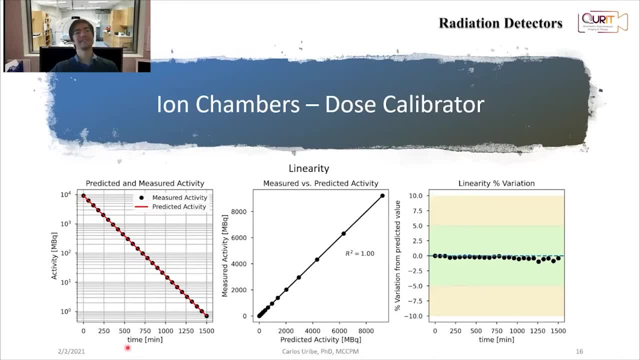 this particular case that i'm showing here. yeah, this is a logarithmic plot, so it follows a line. we see that that predicted activity, based on what we know of the physical decay, and the measured activity is corresponding, and yeah, so there is a very, very little variation in linearity. 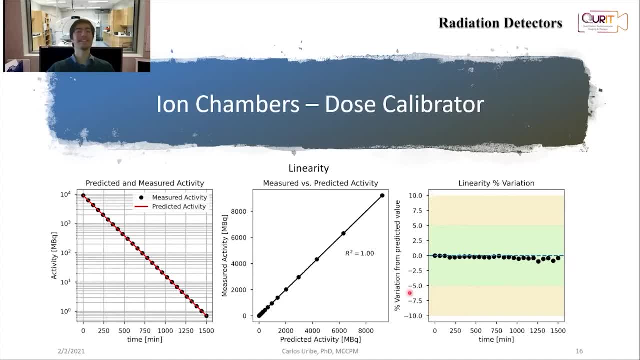 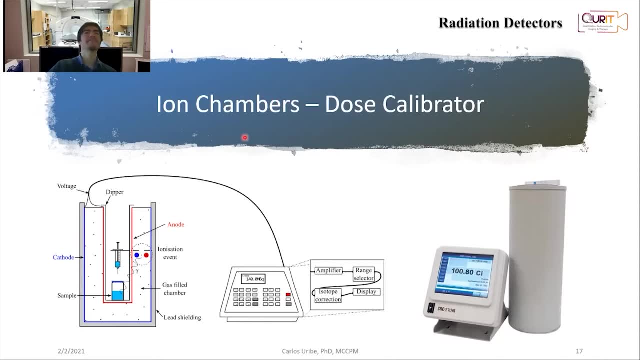 so then we know that that that is accurate. so well, this is how an ion chamber for the dose calibrator looks. so you have the cathode out here, the anode is right here, you have the argon gas inside, so you put your sample inside the dose calibrator. so here is represented by the syringe, or you can put 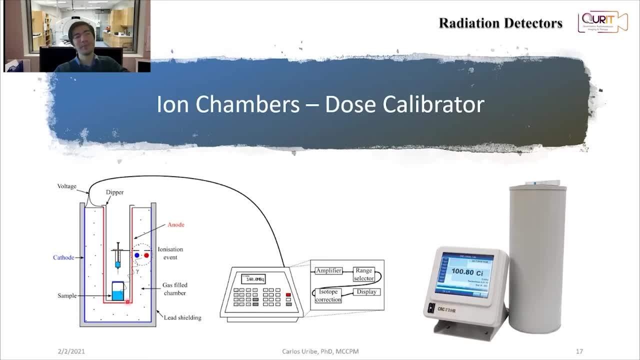 a vial. so look at, those are just this same Stuffanous, rapidly changing回來� n and we kind of you know two different geometries that might cause slightly different number of ionizations. this causes a current when the gas is ionized that the electrometer and the electronics in this device. 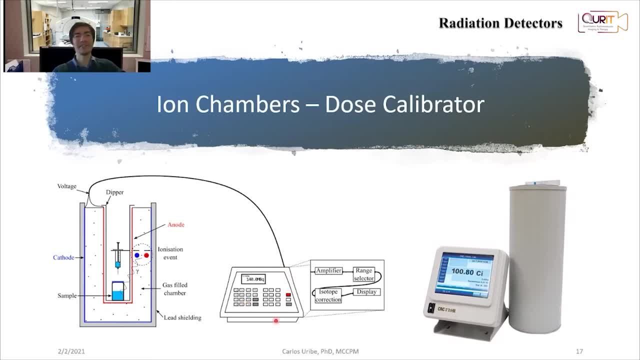 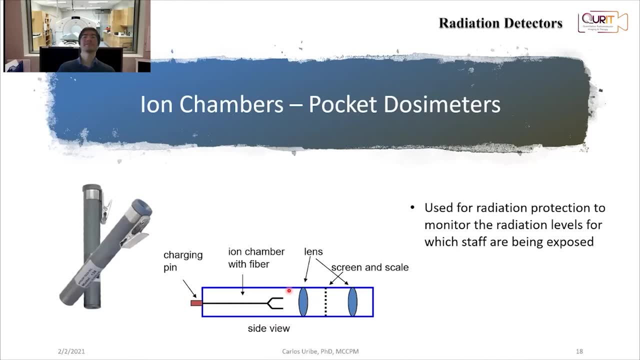 measure and we multiply that current by that calibration factor and then we can, at the end, measure our activity. another type of ion chamber- and again this one is for radiation protection- is something that we call pocket dosimeters, and pocket dosimeters look like this. so the way, okay. 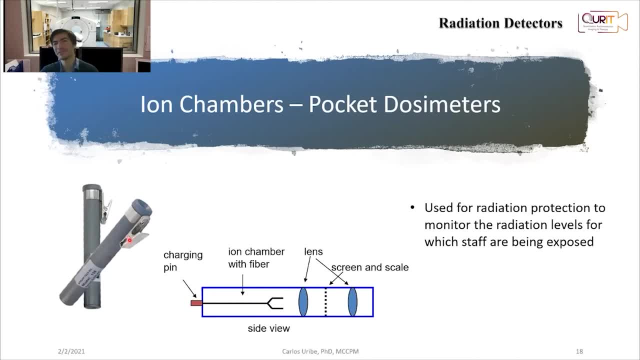 so pocket dosimetries are used to, to measure, to monitor the radiation levels at which staff are being exposed. so so how does it work? so it's basically a capacitor. so in a gas, so you have this capacitor charged, and so you, you, you connect these pocket dosimeters into a 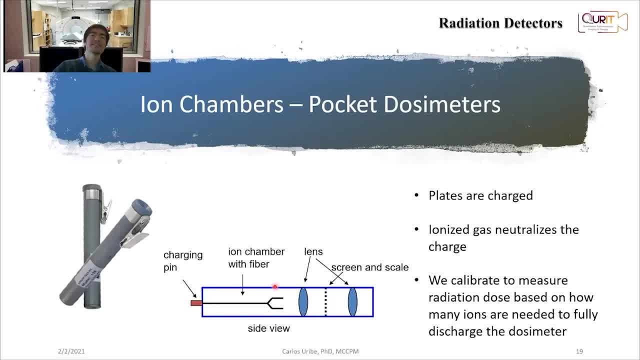 direction A. so the way this works is you: you connect these pocket dosimeters into a, began cleansed and then this comes out. so this is not. it's not the way. now, this is a part of the official that charges this capacitor, but because this capacitor is inside an ion chamber, what's going? 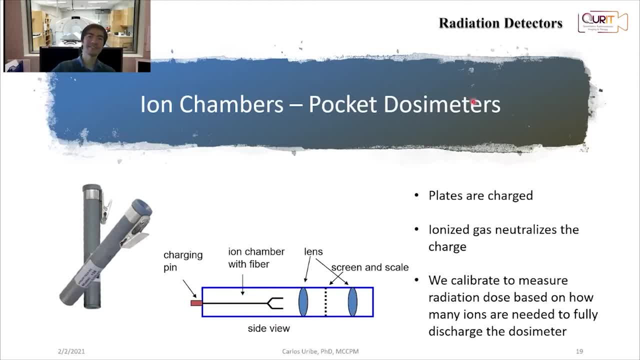 to happen? well, it's inside some gas. if ionizing radiation comes into the dosimeter, it's going to cause some ionizations and then positive charges are going to go to the negative charge plate of that capacitor and negative charges are going to go to the positively charged plate of that. 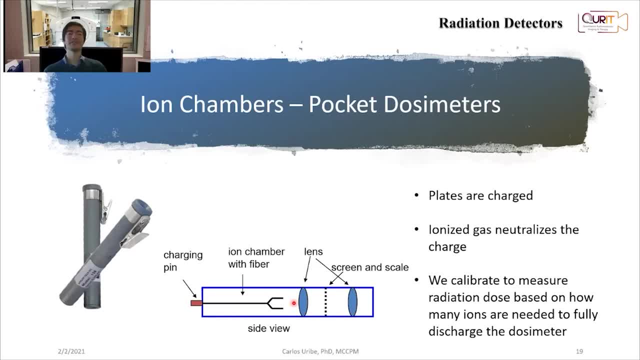 capacitor and as this goes on over time, you start discharging that capacitor. now that this device has a little dial so you can okay. so there's a little window here where you can look with your eyes and there's a little dial inside that's pointing you, so that dial is calibrated to that. 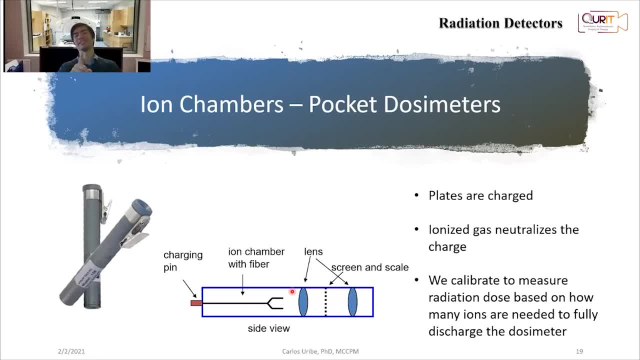 charge of the capacitor. so as the capacitors is discharged, that little dial moves and you can well- there's a scale calibrated to you- present the dose in that that staff member has received. then, once the capacitor is fully discharged, you can again connect the little dosimeter to a device that charges the capacitor. 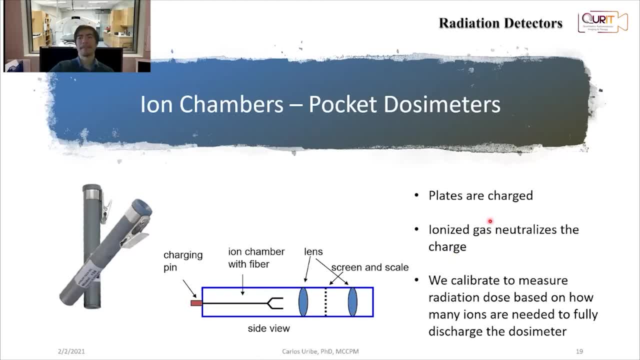 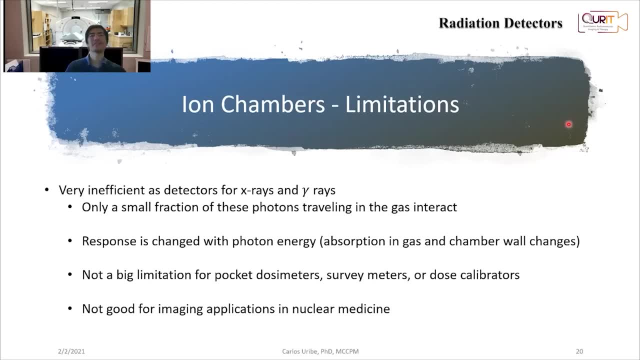 again and then you can reuse it. yeah, so that's basically what i just said. now there are some limitations for the for the ion chambers. one is that they are very inefficient as detectors for x-rays and gamma rays, and well, in a way, yeah, gamma rays and x-rays are more or less 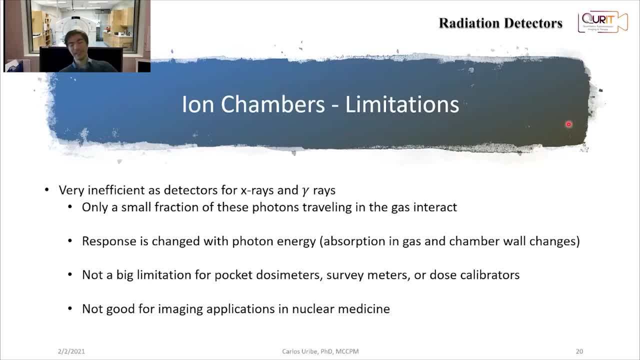 high energy photons. so, coming back to our attenuation coefficients, then, because these gases are not very dense, then the probability of interaction of these x-rays and gamma rays is is small. so only a small fraction of of those photons traveling in the gas will actually interact with the gas. and now the response is also changed with photon energy and what you can think. okay, now, 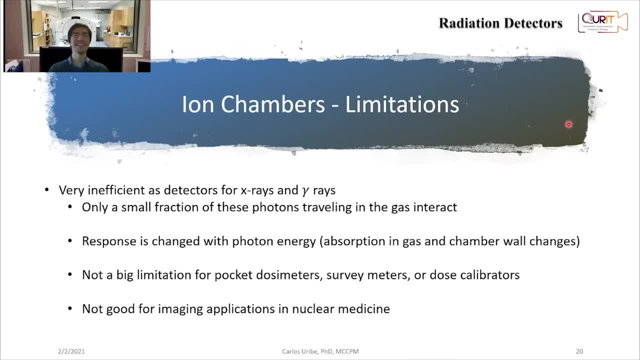 these chambers have a wall so, depending on the energy of the photons, maybe you end up getting some ionizations caused by actually interactions from the photons on the wall- not really necessarily on the gas, but then that changes as well with the energy of the photons. this is not a big limitation. 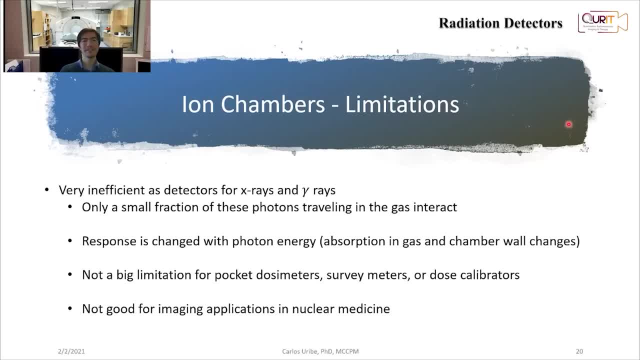 for pocket dosimeters or something like that, but it's not a big limitation for pocket dosimeters or segment meters or those calibrators, however, but it's of course, not good for imaging applications in nuclear medicine, because you for me to be able to create a good image, we need to be able to detect. 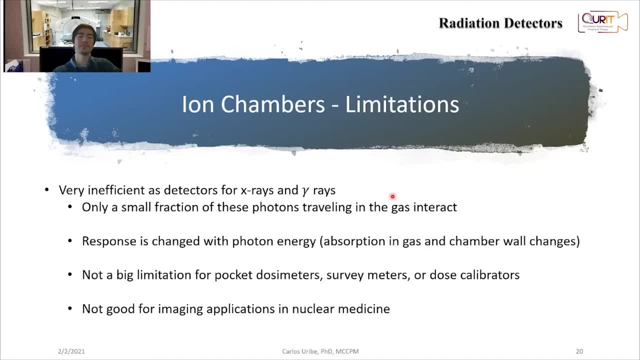 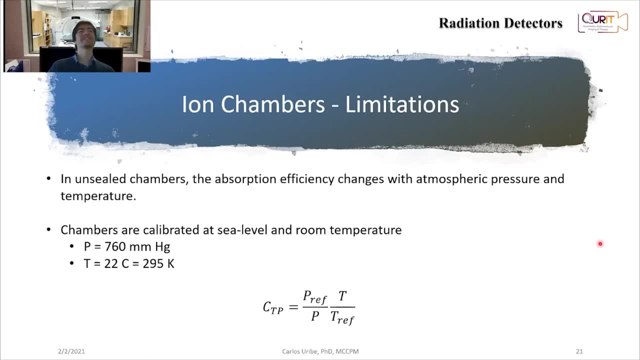 a lot of a big number of gamma rays or or x-rays. there's another limitation. so if you are using unsealed chambers- those are the ones that are exposed to atmospheric pressures- then there might be differences in absorption efficiency. for example, you are at sea level, compared if you go up a mountain. 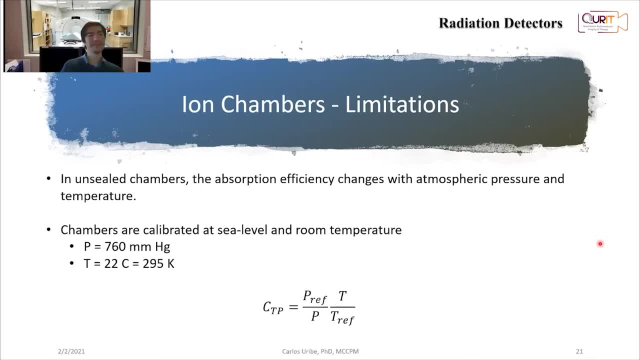 and then there's differences in that pressure: if you are at 22 degrees celsius, which would be room temperature, if you are at 40 degrees celsius. so these chambers are calibrated for sea level and room temperature, but if you are doing your measurements at different, in different, 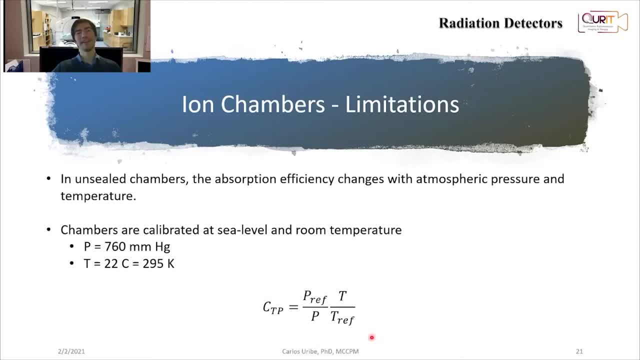 conditions, then there has to be one calibration factor that also needs to be taken into account. that is typically calculated by taking the reference pressure. it will be this one, divided by the pressure at which we're taking the measurement times, the temperature at which we're taking the measurement. 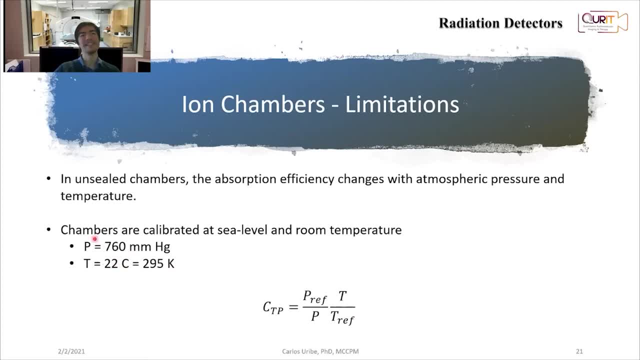 over the reference temperature, which is 22 degrees Celsius. I'm gonna edit this slide just to make it explicit that this is P? ref and T ref, because now I'm seeing that there might be a confusion there. So that's ion chambers. 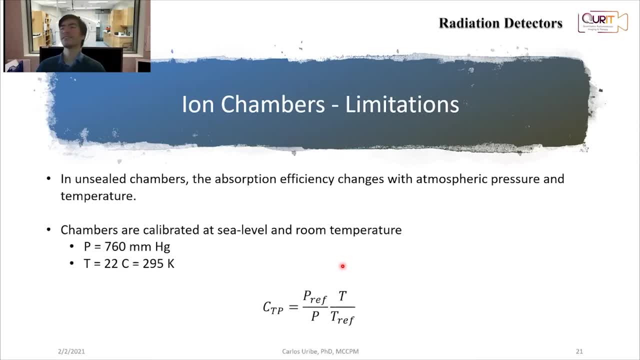 Now I think there's some people asking why they put argon, not other type of noble gas. This one, for me, is hard to analyze. I'm gonna use argon. Armando, do you know why they would use argon instead of another noble gas? 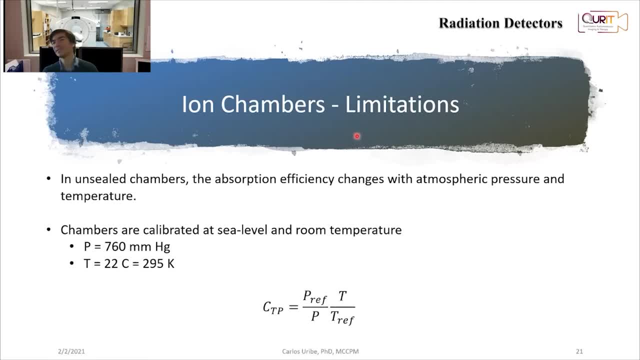 Yeah, what is specific about- So they use a noble gas just because, of course, you want this argon to remain being argon for as long as possible. But I don't really know exactly why would argon be the gas to choose? 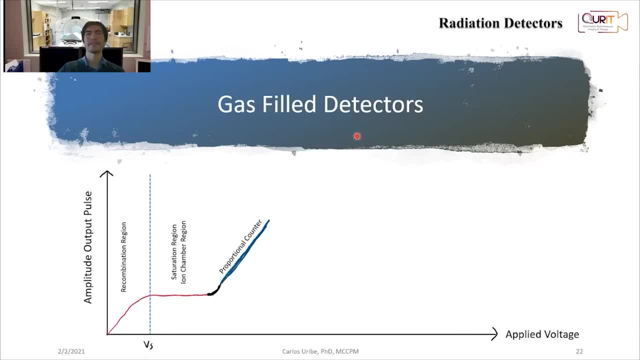 So I'll do some investigation about that and I'll get back to you. Okay, so let's keep increasing the voltage. Now we're in the ion chamber region. We can keep increasing, increasing, increasing the voltage, And then we get to a region that we call. 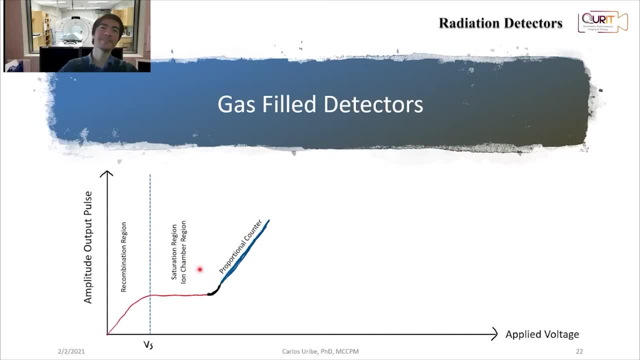 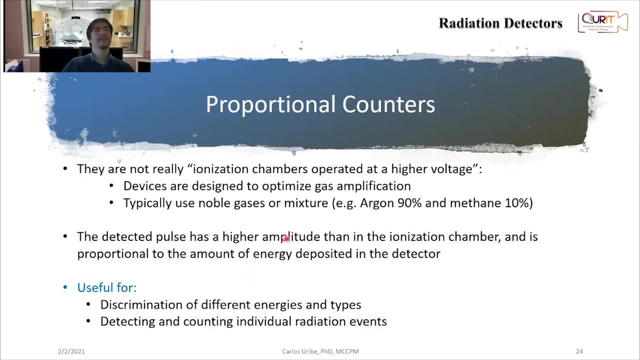 the proportional counter region. So what this is happening is, as you increase the voltage, your output pulse starts going high and higher. So well, although you would think that they might be just ionized energy chambers that operate at higher voltages, it's not really necessarily the 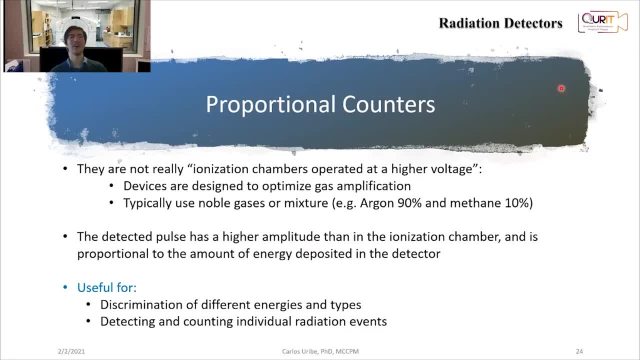 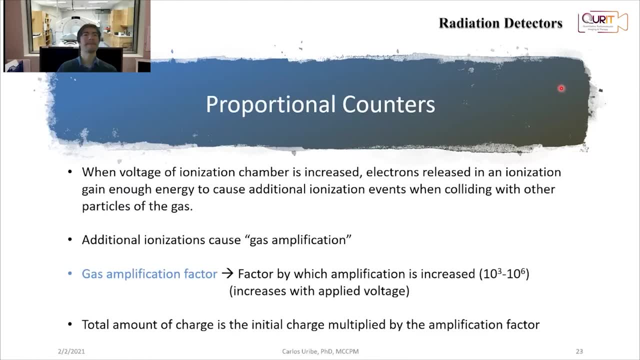 case, They're actually designed to optimize what we call the gas amplification. Sorry, I skipped one slide. Yeah, so when the voltage of the ionization increases, okay, we now increase this voltage. what happens is that what we what is known as the gas amplification. And then you can think about defining a factor. 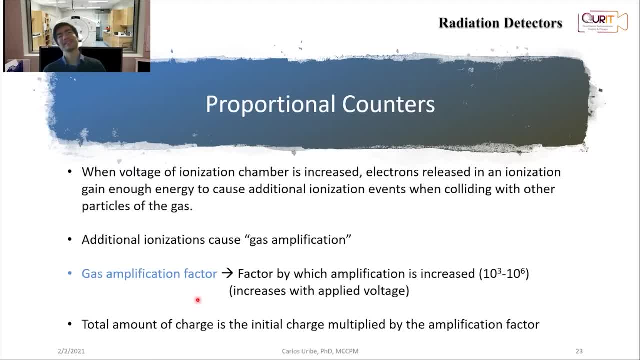 which is the gas amplification factor. that is the by which that amplification is increased. I mean typically in proportional count. it goes from 10 to the three to 10 to the six. It goes, it grows and grows as the voltage is increasing. 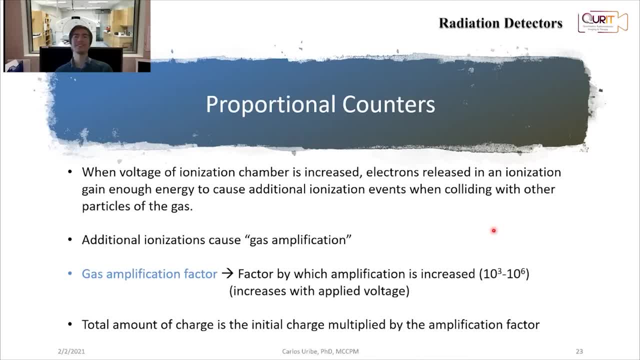 So if in the ion chamber you had one ionization, maybe in this proportional counter that one ionization is gonna become 1000 ionizations. So you don't measure the total amount of the initial charge. You now measure that total charge after the amplification. 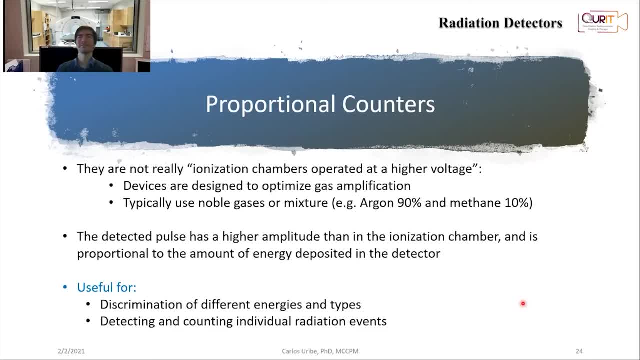 But what I was saying when I go. they are not really just ionization chambers that operate at high voltage. They are actually designed to optimize that gas amplification And they typically use noble gases or mixtures. One example is argon 90% and methane 10%. 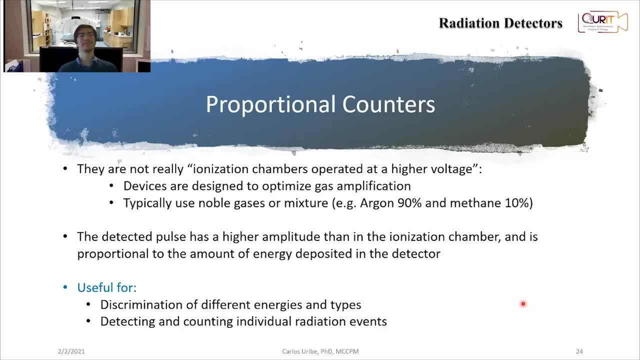 would be a combination that would be useful. Now, this pulse is, of course, higher than the gas ionization chamber, And it's proportional to the amount of energy deposited in the detector, So it's very useful if you wanna discriminate different energies and types. 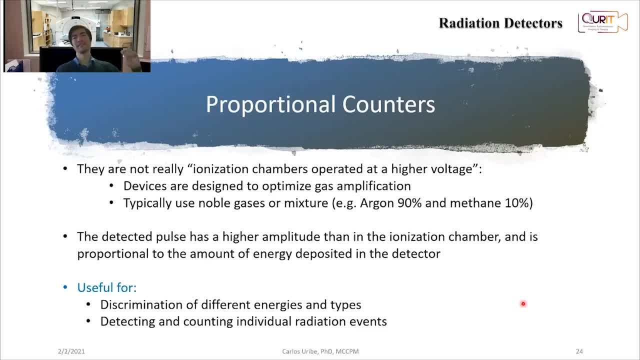 because you bring your detector, you have a height of your pulse When, let's say, you have a small amplitude pulse. if that energy is low, you get a high amplitude pulse. if your energy is high, You get a high amplitude pulse if your energy is high. 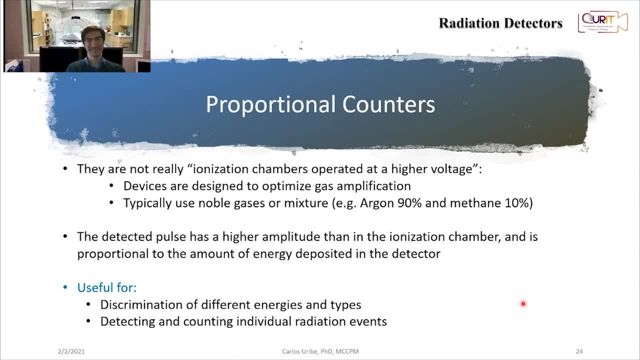 You get a high amplitude pulse if your energy is high, So you are able to distinguish more or less when you have a low energy radiation than when you have high energy radiation, And it's also useful for detect and discount individual radiation events. They are still, however. 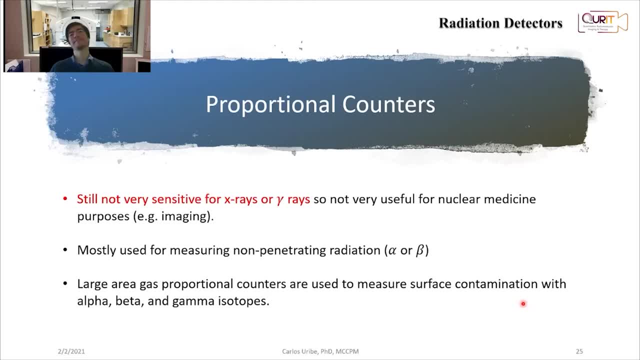 not very sensitive for X-rays or gamma rays. So again, they're not very useful for nuclear medicine besides, probably just radiation protection. in the clinical environment They're mostly used for radiation protection. They're mostly used to measure non-penetrating radiation. 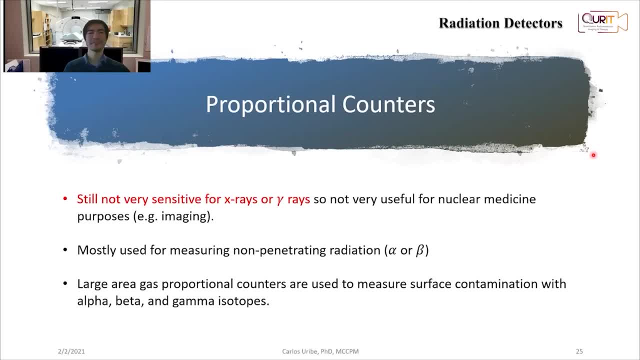 such as alphas or betas, And we haven't fully talked about this. We're gonna get that to it later- but alpha particles and beta particles can be easily stopped with, maybe with a very thin piece of paper, for example. So that's what we mean, that this is non-penetrating radiation. 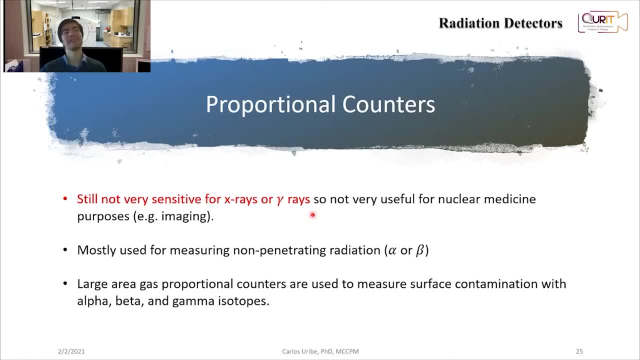 So if it's outside of your body, well, it's hard for it to enter your body, unless maybe you just swallow it or something like that. When we have large area gas proportional counters, they are typically used to measure surface contamination, when typically that contamination is caused. 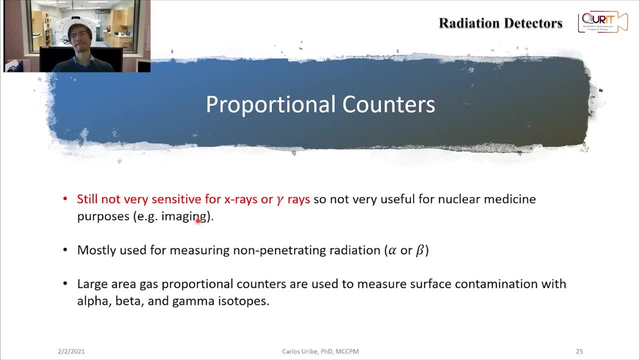 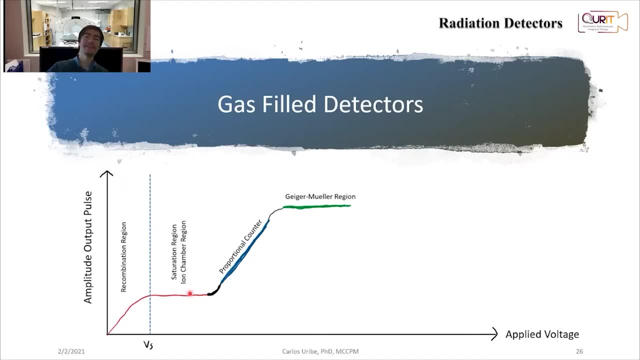 by alpha, beta or gamma isotopes. And then let's keep increasing the voltage to that gas chamber. So you start increasing to the proportional counter. You start going up, you keep going up, you keep going up. but then you Now let's restrain. So right now let's drawers. sometimes I guess, sitting on my stage, maybe three or four clothes in the trash. 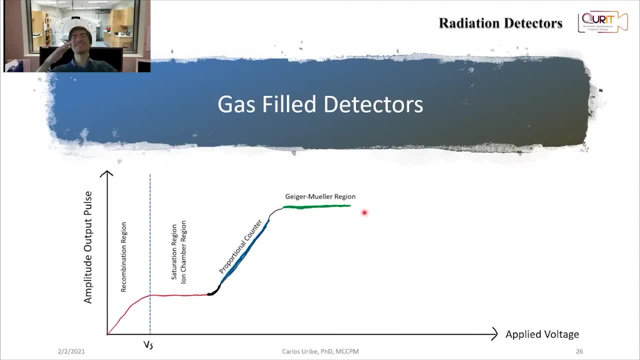 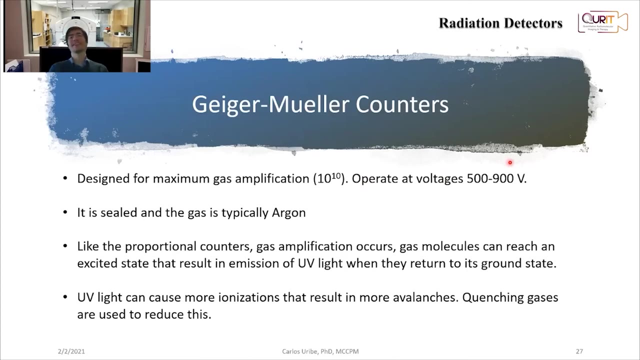 you get to this region that is more or less flat. it's not exactly horizontal. it has a little bit of a slope, but it's not a big slope, and this is what we call the Geiger-Müller region. so what is that Geiger-Müller region? so Geiger-Müller counters, which is the name of these. 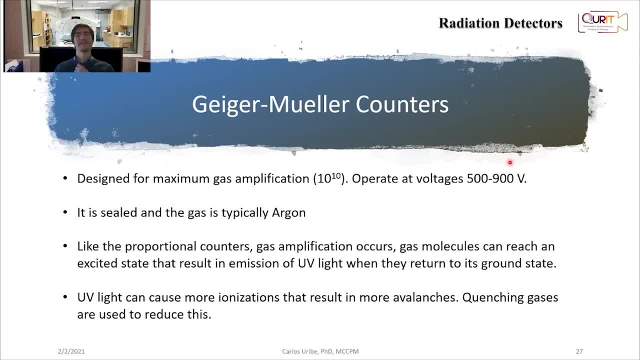 detectors operating in this region are called. this is a region that is typically between 500 and 900 volts between the electrodes and they're designed to have the maximum gas amplification as possible. so remember, before we were in that proportional region we had an amplification. 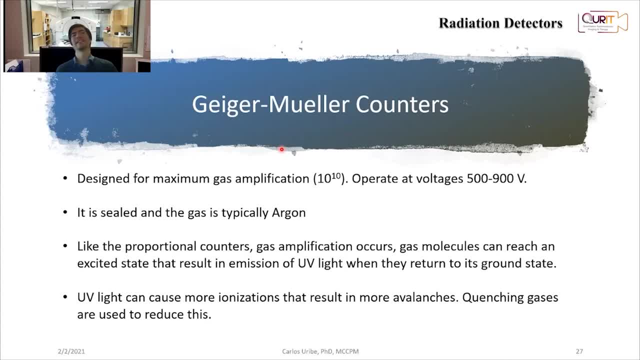 between 10 to the 3 and 10 to the 6. now in Geiger-Müller counters it will typically go up to 10 to the 10. a factor of 10 to the 10 of amplification. Geiger-Müller counters are sealed. 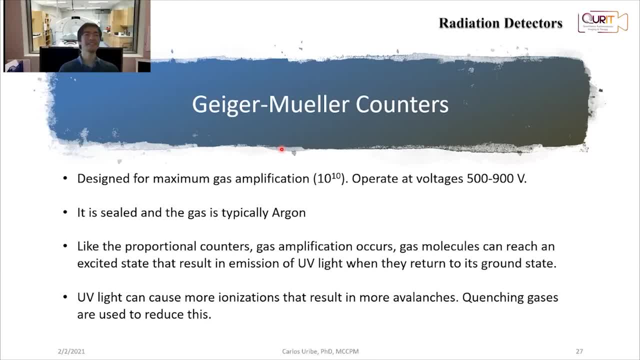 again typically filled with argon. now these proportional counters have this gas amplification, but then the issue is that gas molecules can also become excited, and if these molecules are excited, then when these molecules come down to their ground state, we have an issue, and is that they emit. 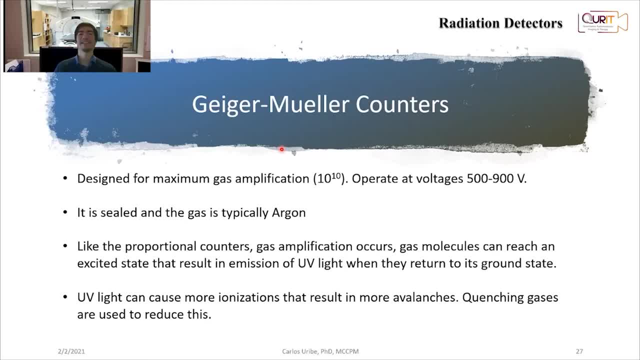 they typically emit ultraviolet light, and if you have this ultraviolet light, then what this causes is that maybe this ultraviolet light is going to cause some other ionizations by itself, and then this is just resulting more and more avalanches, and an avalanche is you receive one particle and this amplifies and you receive one particle that just 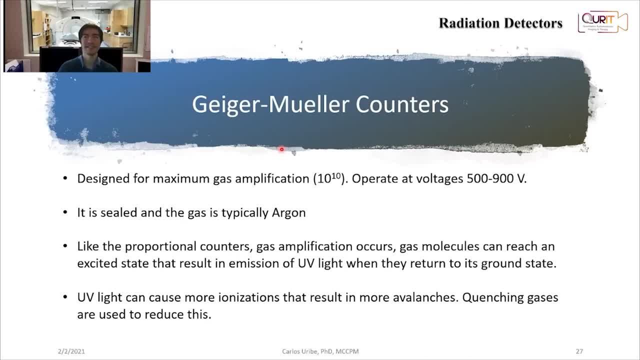 gets amplified and amplified in different ionizations. so because there's this UV light that can cause more ionizations and then this is just resulting in more avalanches, and then this just can't be up to a state, but it just keep, can't keep going when it's amplified. it can't be. 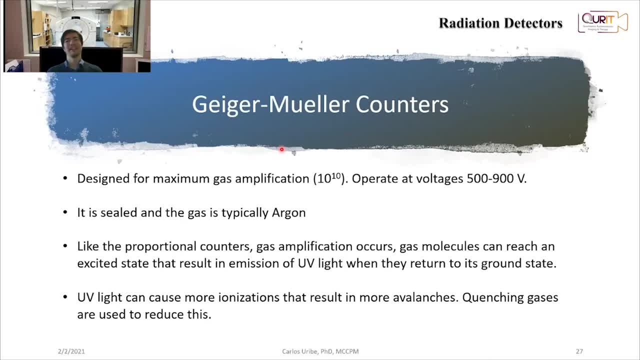 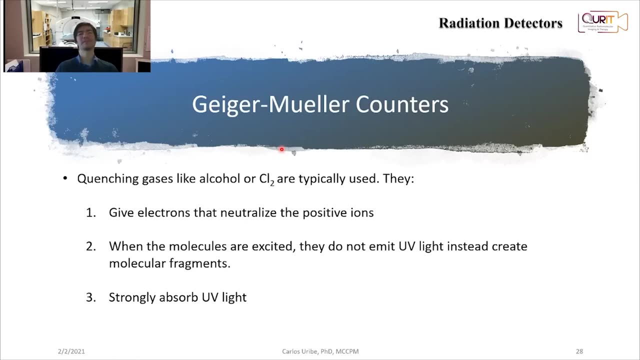 to stop those avalanches caused by this UV light And to do that we use what is called quenching gases. So quenching gases basically will stop the avalanches. So quenching gases can be well common. quenching gases can be alcohol or chlorine are typically used. So what are they doing? 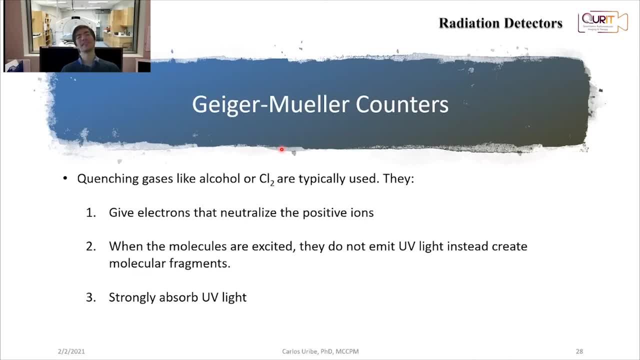 One. these quenching gases give electrons that neutralize the positive ions. So you have an ionization. you have positive ions, you get negative ions. The negative ions will move much faster towards the positive charge of the electrodes. The positive ions are heavier. 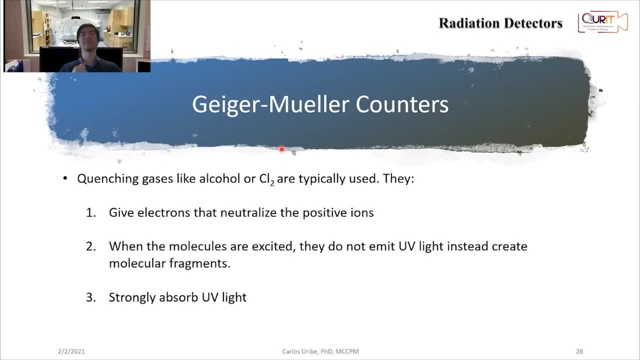 so they move slowly. So in that process of moving these positive charges, these quenching gases will share some of their electrons, So then that positive charge is going to be neutral again. Now these quenching gases, the molecules of the quenching gases, are excited. One of the things that is very good about is that. 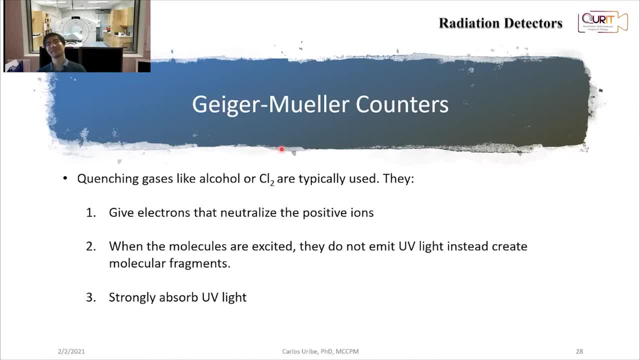 they do not. they're not going to come back to the ground state and be in UV light. They will instead kind of create molecular fragments. They're going to fragment themselves. And a third characteristic is that these quenching gases strongly absorb UV light. 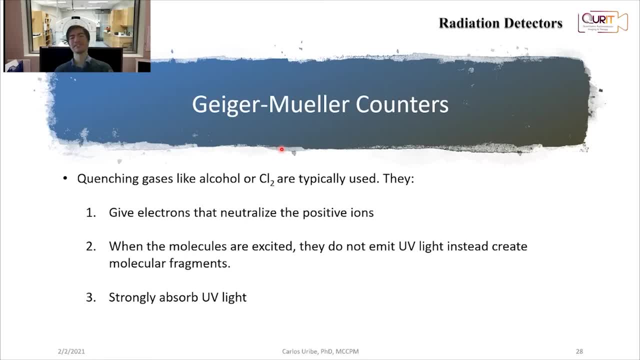 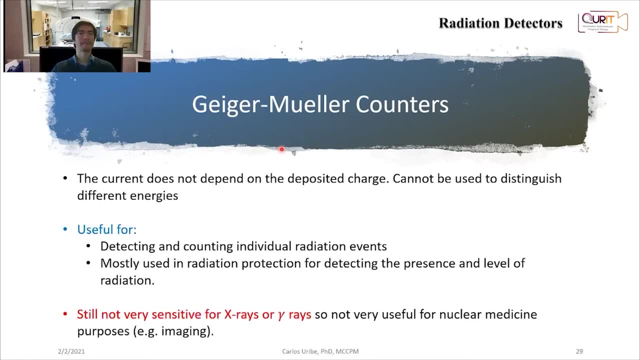 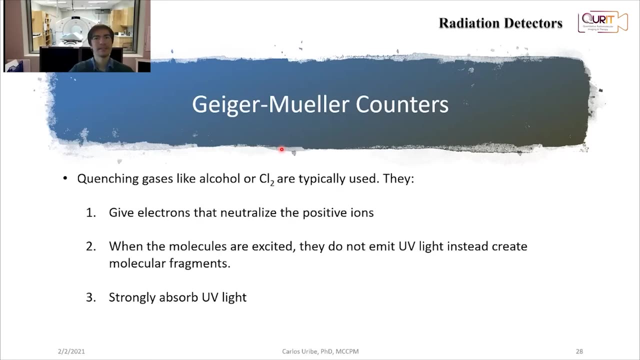 So then, these UV light, instead of causing more ionizations, it's just going to be completely absorbed by the quenching gases and that's going to stop the avalanche. Now, okay, I'm going to say it here because I'm not sure if I have it. 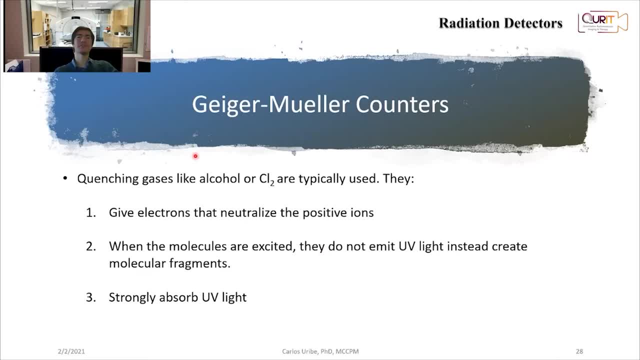 Typically when organic gases are used, for example alcohol, what happens is as they well, when they have these molecular fragments, they're not going to become what they were before. So as time goes by, then you're going to start losing your quenching gas. So after a while it needs to be replaced. 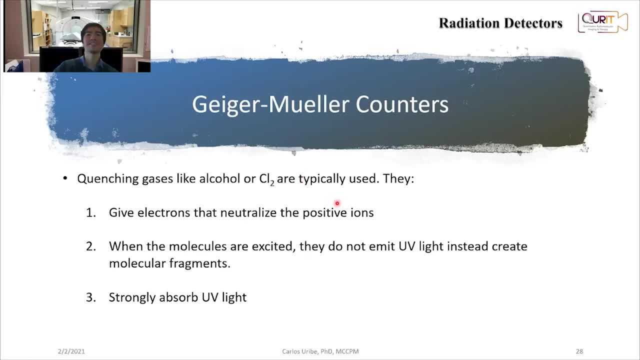 But when chlorine two is used- chlorine use- these molecular fragments actually recombine into chlorine molecules. So then these detectors will last for much, much, much longer. After they disintegrate those molecular fragments they can come back together. So this is a very, very, very 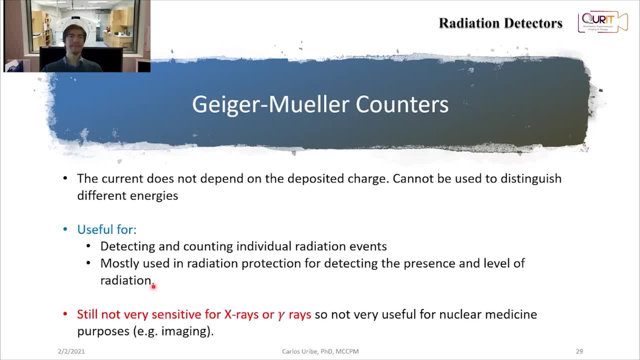 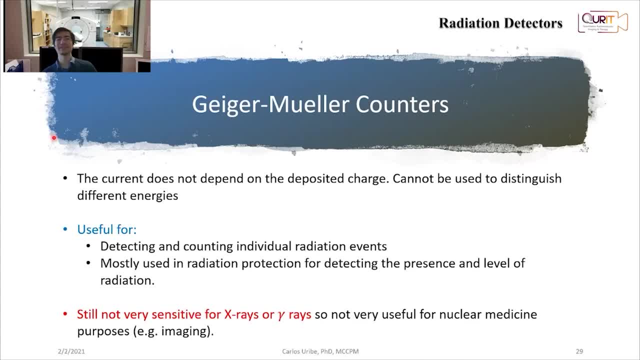 Oberhart, eat again as sort of a summative and counting individual radiation events. You can count. That's why they're called Geiger-Muller counters. You'll know if you had one event or three events coming. They're mostly used again in radiation protection. 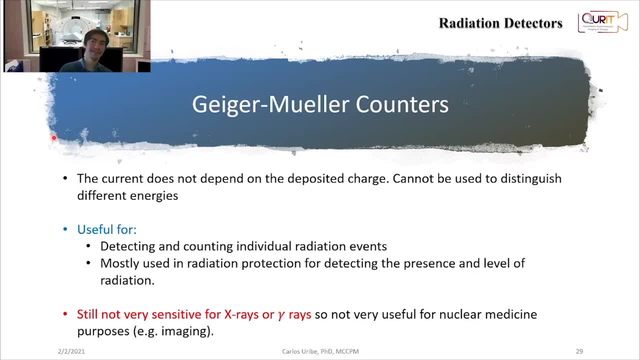 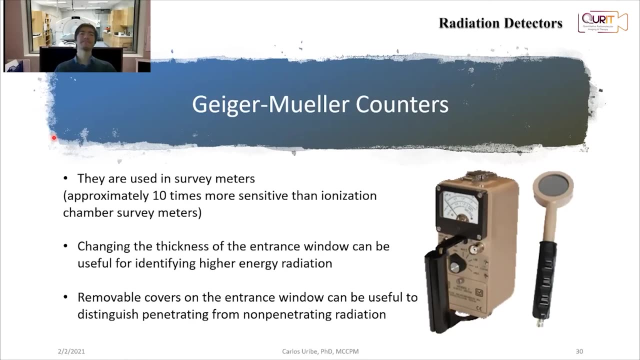 for detecting the presence of radiation, Still not very useful for nuclear medicine purposes. So again, they're not very sensitive for x-rays or gamma rays. Geiger-Muller counters are also used in survey meters, So they are survey meters that are approximately 10 times more sensitive. 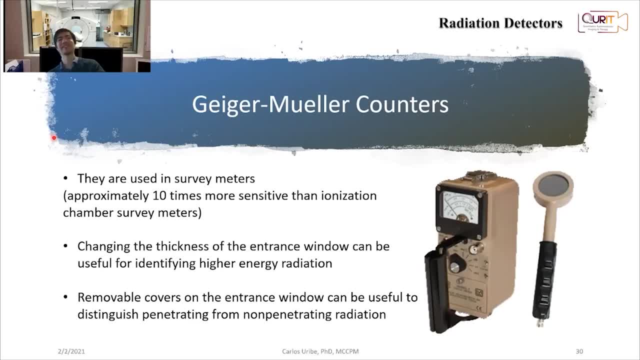 than the survey meters that work with just the ionization chamber region, Changing the thing. Okay, so if you look at this device I'm showing on the right- and this is what we call typically a pancake, and devices because of the shape. 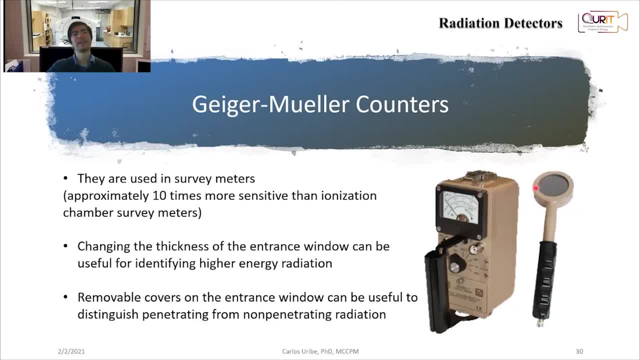 that you have in the detector. Well, if you change the thickness of the entrance window, you can identify a little bit the energy of the radiation, And because thicker I mean low energy radiation will probably not be able to travel through a very, very thick window. 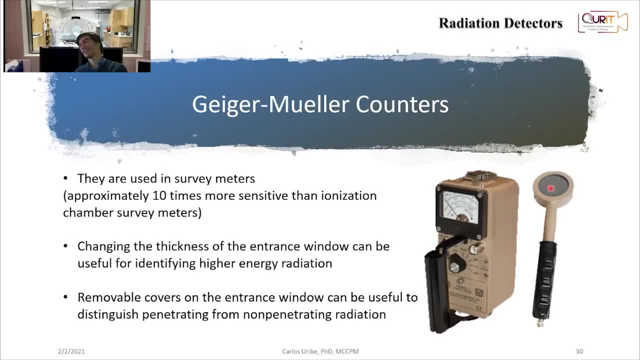 And something that it's used to, for example, distinguish gammas from. if you have some contamination and you wanna know if that contamination is caused by a beta-emitting isotope or by a gamma-emitting isotope, you can use this. 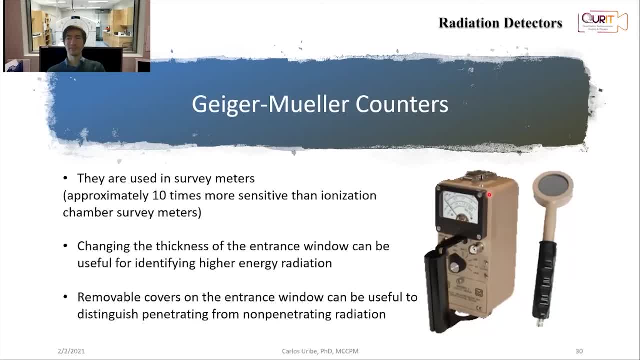 One of the ways that is done is because betas are easily stoppable. You put like a little plastic on this entrance window And if you don't measure anything- but then when you take the window you have some measurements- you know that those are caused by betas. 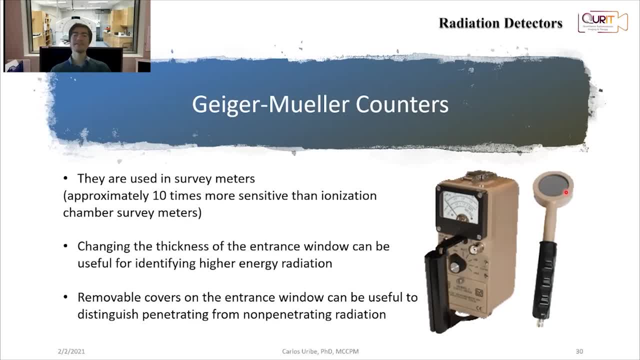 It's just that the plastic is stopping your betas Gammas. well, the plastic is basically transparent to the gamma. so if you put the plastic window and you still see exactly the same as when you didn't have the plastic window, you will know. 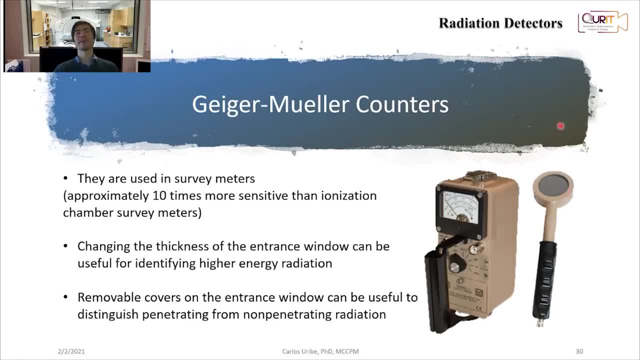 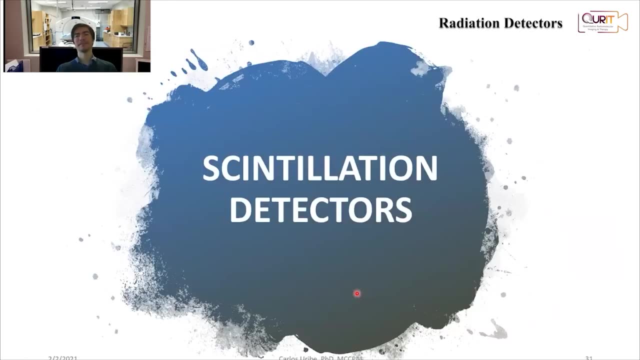 that that contamination that you have there, it's caused by a gamma-emitting isotope. Yeah, so that's how it's useful to identify between penetrating and non-penetrating radiation. Are there any questions up to this point? Well, scintillation detectors. 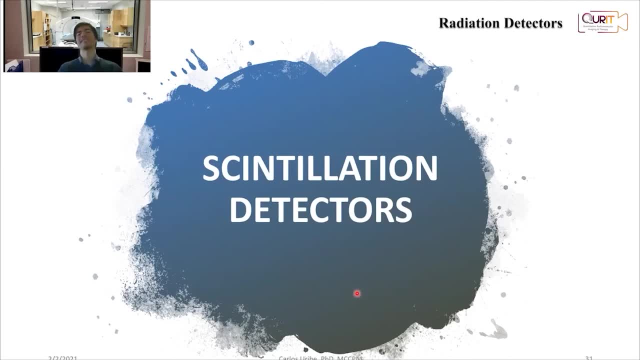 I'm not gonna go into details. I just want you to know that it exists. Armani is gonna give a very, very nice lecture of these and we're gonna start looking into some mathematical measurements that we can do, but I'm not gonna go into details. 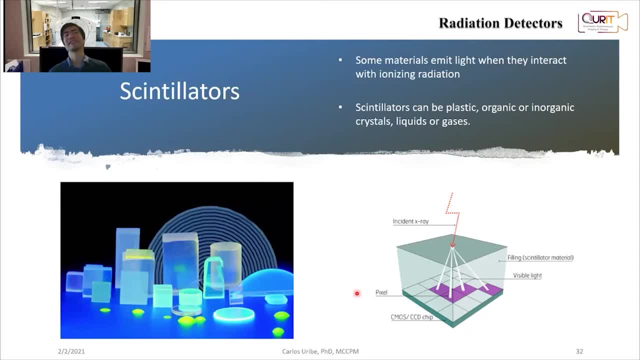 I just want you to know that it exists. But just as a quick introduction, these are just some detectors that when they interact with radiation, they emit some light, And scintillators can be plastic, can be organic or inorganic crystals. 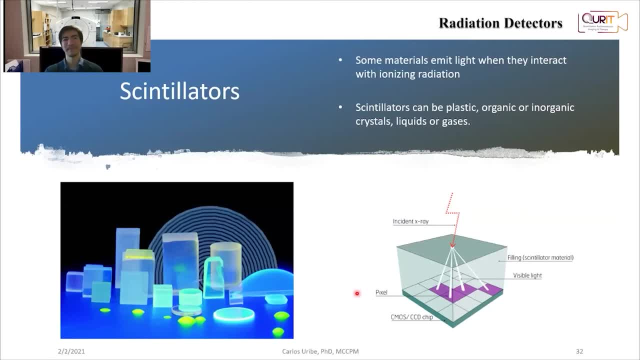 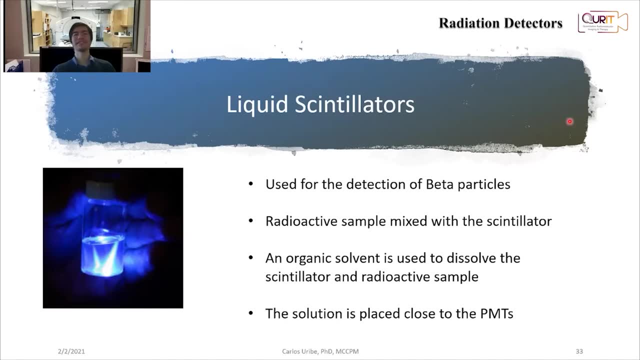 We can have liquids or we can have gases. Liquid scintillators, for example, what I'm showing you in the left. they're typically used for beta particle detection. You mix the radiation with your liquid scintillators. you mix the radiation with your liquid scintillators. 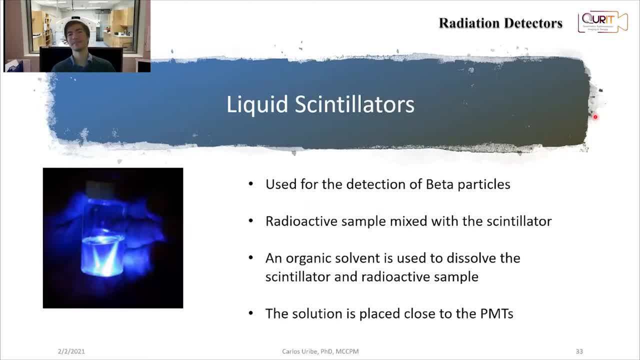 you mix the radiation with your liquid scintillators and then they emit light, So that organic solvent will dissolve the scintillator in a radioactive sample, and then we can place this solution into a detector to just count the light and we'll be able to quantify the same. 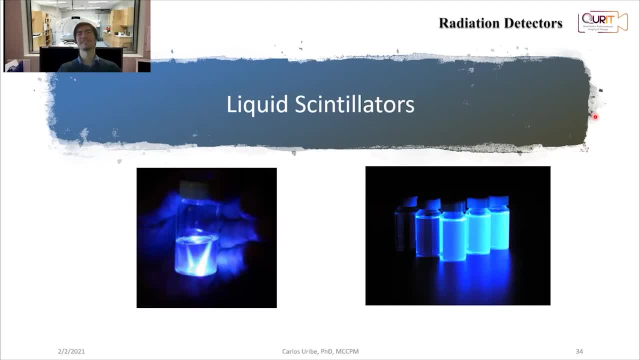 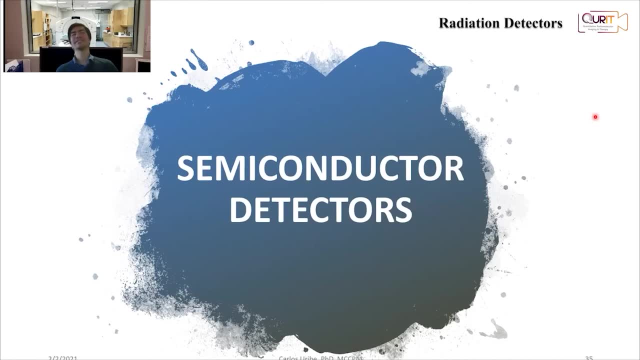 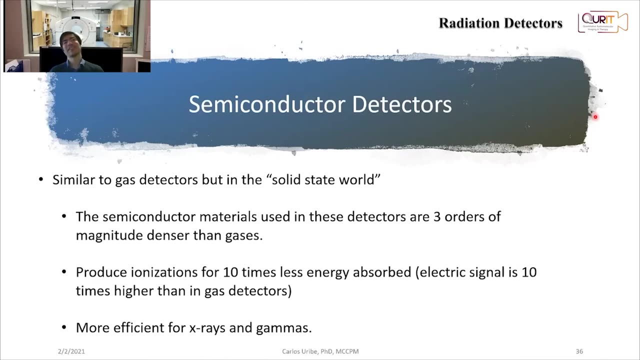 Well, just so you know. but stay tuned, The next lecture is focusing more on scintillators. Lastly, let's talk a little bit about kind of newer technologies which are semiconductor detectors. Semiconductor detectors, you can think is similar to the gas detectors that we just talked about. 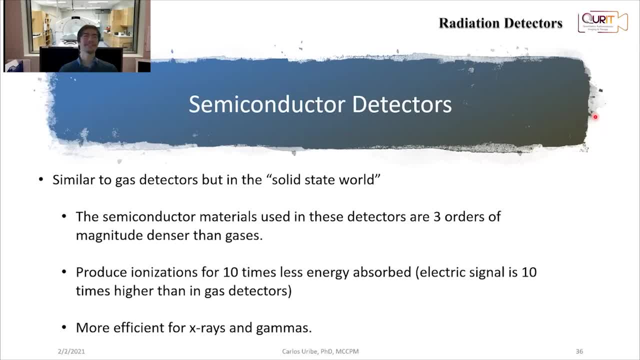 but in the solid state world. So now think about, okay, when you had a gas and we said, well, the gas is definitely not dense enough to really stop all the gammas. Now, this is solid, this is in the solid state. 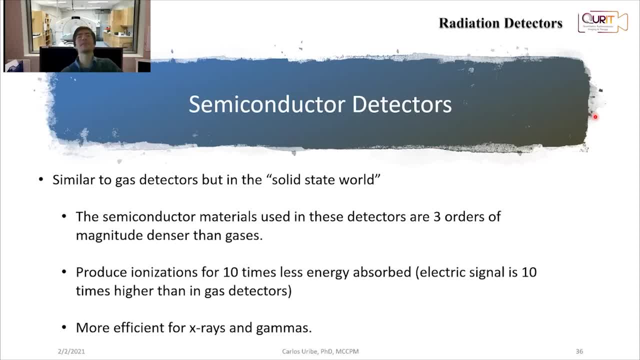 These are solid detectors So they have a magnitude of around three times. there are three orders of magnitude denser than gases. So if they are denser than gases they can produce ionizations for 10 times less energy. So the electric signal that you can measure. 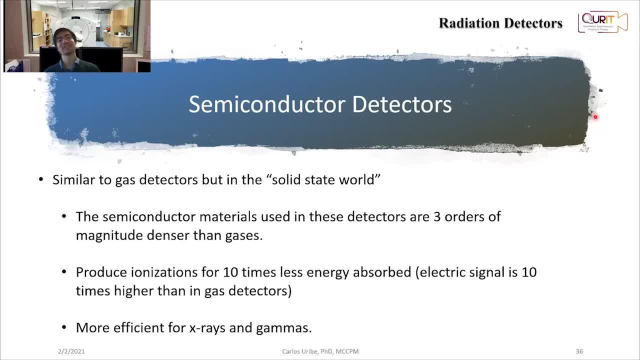 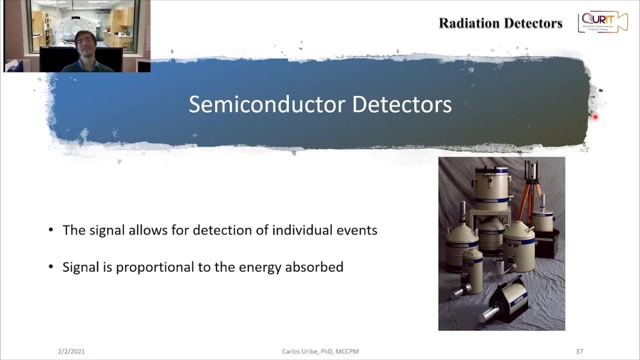 becomes basically 10 times higher than in gas detectors. So now they start becoming more efficient for X-rays and gammas, which was the limitation from all those gas detectors that we discussed a moment ago. Now the signal from the detectors: they do allow for the detection of individual events. 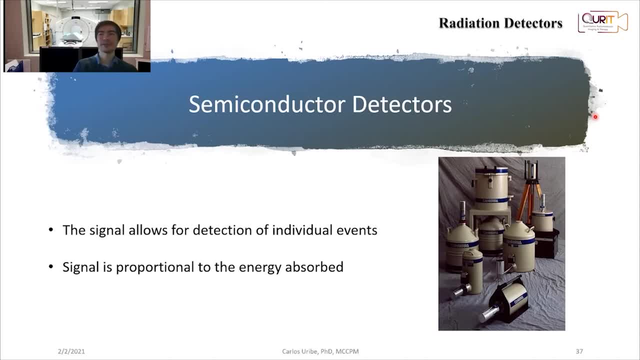 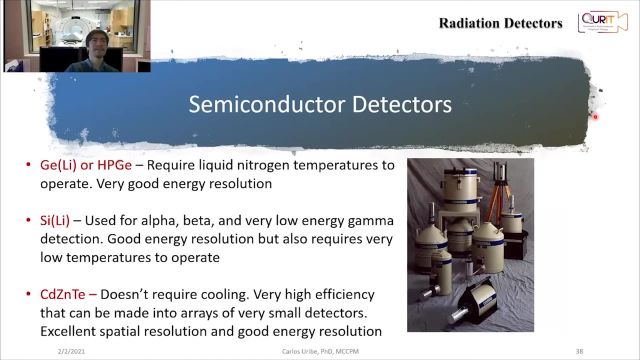 and the amount of the signal that we collect, so that pulse of energy is proportional to the energy absorbed. So if there's a higher energy photon or a lower energy photon, we'll see a difference in the electric pulse that it generates. So we started looking, okay, tip. 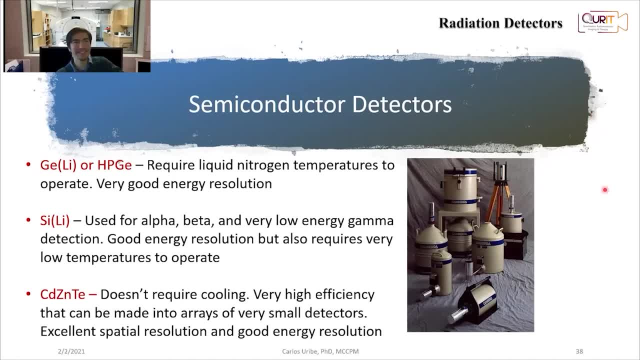 these are typical materials of semiconductor detectors. So some semiconductor detectors are made of germanium, Some others are made of silicon, And they're very well. they're very good. It's just that they have a very big limitation, And it's just that they require liquid nitrogen temperatures. 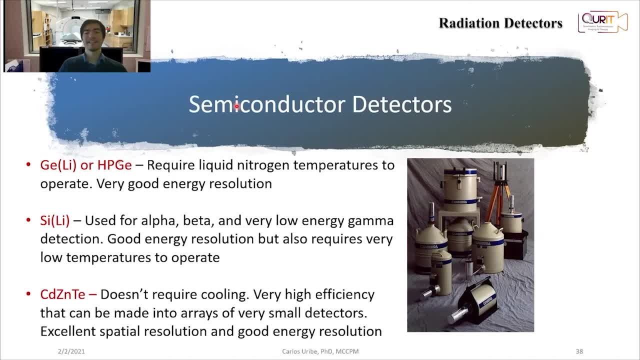 to operate. The reason for this is that at thermal- okay, at room temperature, basically- they do conduct. they conduct electrical currents, So then that adds noise to. well, there's background noise in your current, So you don't want to use that noise. 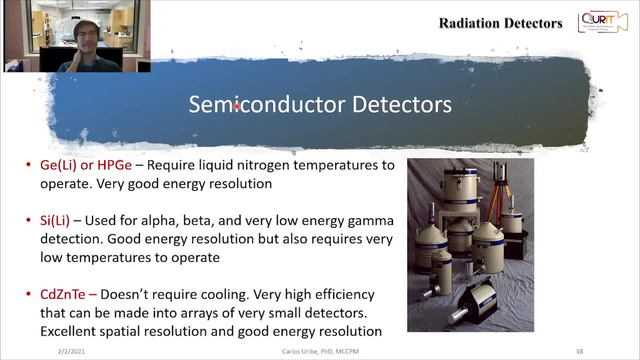 It just contaminates your measurements. Now, when we think about germanium and silicon, by itself they can have end up having some impurities. And when you have some impurities in these, in these solid state detectors, these impurities, 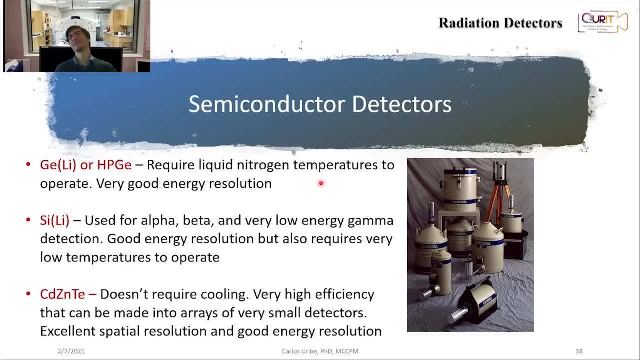 create what's called an electron trap. So if you have an ionization event and these ionization event removes electrons from some atoms, instead of us being able to measure that electron with an electric meter, these contamination inside the crystal, the lattice of these crystals, end up trapping. 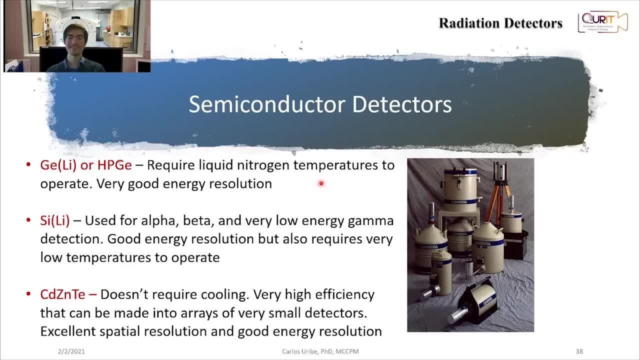 those electrons and then we don't see it. So this makes us lose energy. Sorry, lose, lose, lose energy, some of those electrons that we should be collecting So to solve those problems of those impurities people have tried to then maybe create. 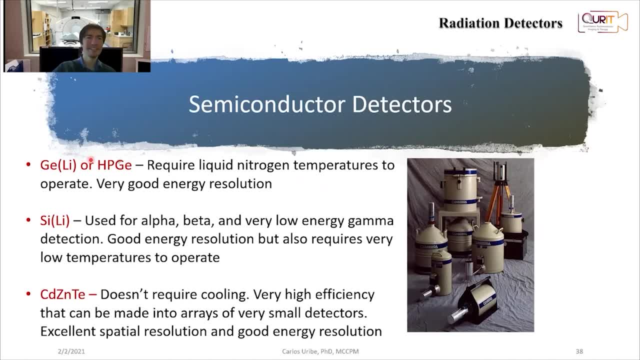 a very, very high purity crystal, And that's what HPGE stands here. So these will be high purity germanium, So that germanium is very, very, very pure. then we will be able to reduce the effects of those impurities causing those electron traps. 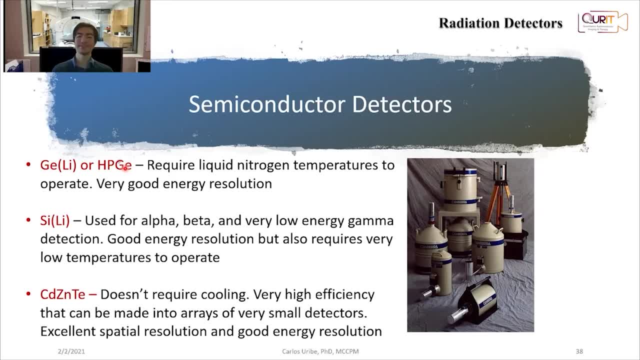 However, doing a high purity germanium crystal is very, very expensive. So well, it's expensive. it's being used, though, but it's expensive. So another option to deal with those impurities in the crystal that are taking some of our electrons. 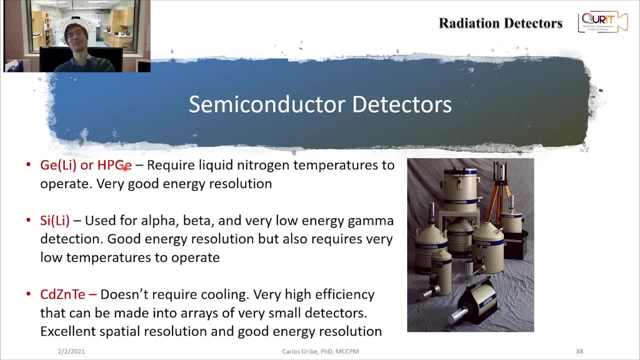 is by introducing impurities that do the opposite. Those impurities will donate electrons and that's why, for example, we have lithium. So that's why you have here germanium with some lithium, silicon with some lithium. So we're, in a way, trying to compensate. 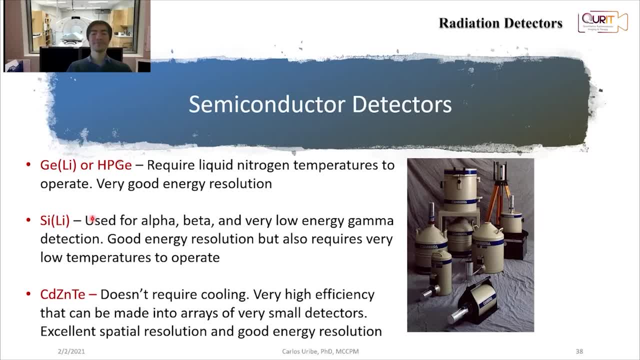 for those impurities by adding lithium. And what lithium is gonna do is that it's gonna give us some electrons to compensate for those electrons that those truck will be losing. Silicon, okay, yeah, Germanium detectors have very, very good energy resolution. 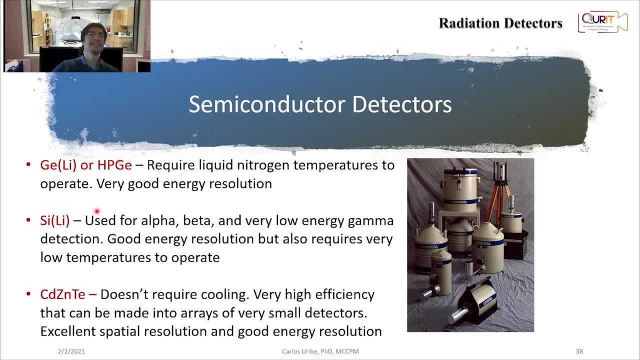 We're gonna see a little bit graph in a moment. Silicon are typically used for alpha, beta and very low energy gamma detection, So they have good energy resolution, but they also require very low temperatures to operate. Now, germanium: they have an even higher limitation. 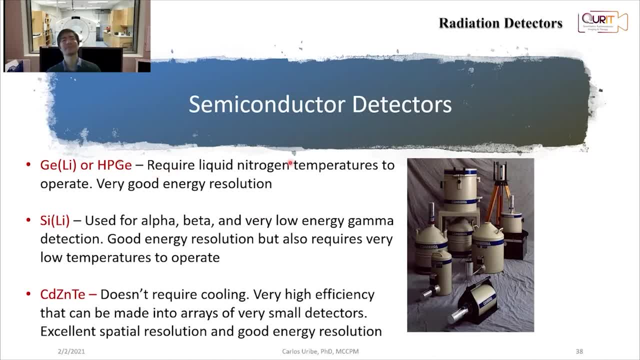 is that they don't only really require liquid nitrogen to operate. they also require to be stored at very, very low temperatures, or your detector is just gonna damage Silicon. you can still store it at low temperature, Sorry, you can still store it at room temperature. 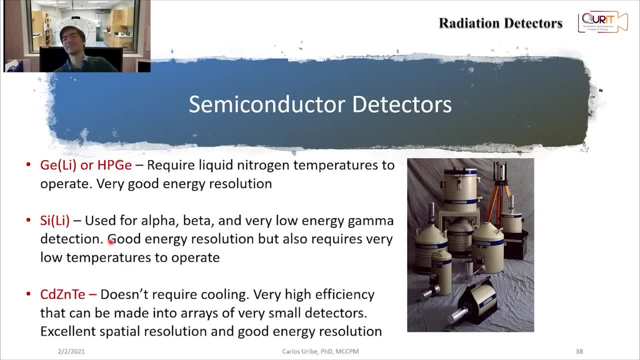 but if you want to make the most of it, it should still be stored at very, very low temperatures. Now, in recent years, to address these issues, people found out these new type of detectors, which are called cadmium zinc telluride. 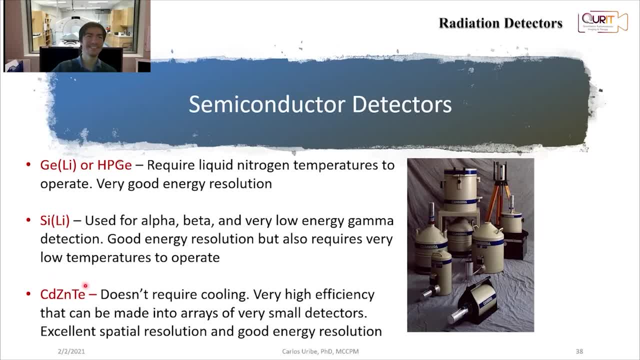 what we just refer to them as CZT, and the main advantage of these detectors- again, they're solid-state detectors, but is that they don't really require cooling. They are very efficient. Okay, so they can operate very well at room temperature. 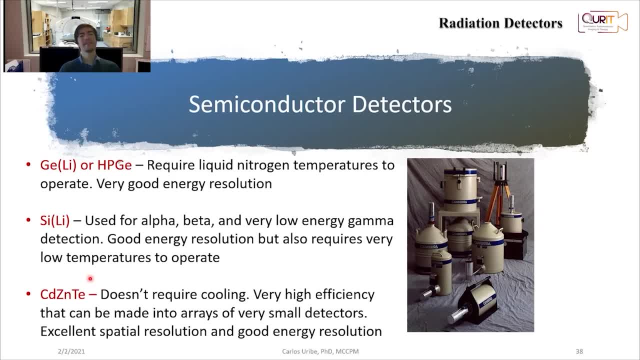 and that's a very, very big advantage. And they can be made into small arrays of detectors, into arrays of very small detectors. So it's really hard to make a very big crystal of CZT, but they found applications when arrays of 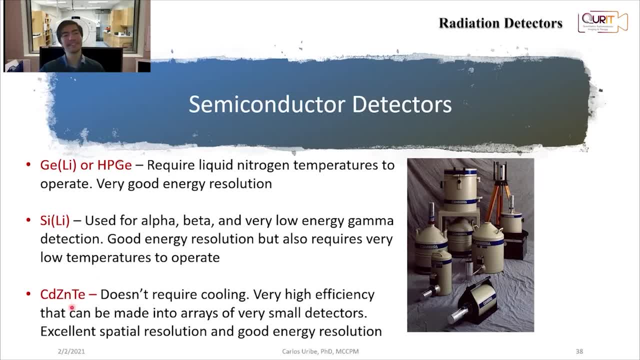 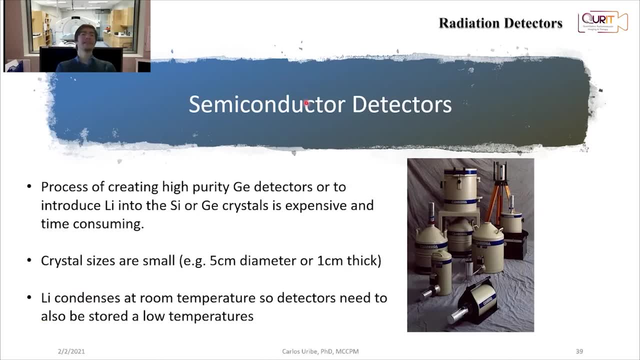 arrays of small detectors can be used. They have excellent spatial and good energy resolution. but we'll look into those details as we keep going. Okay, so, yeah. so the introduction, either the growing of high germanium detectors or the introduction of those impurities. 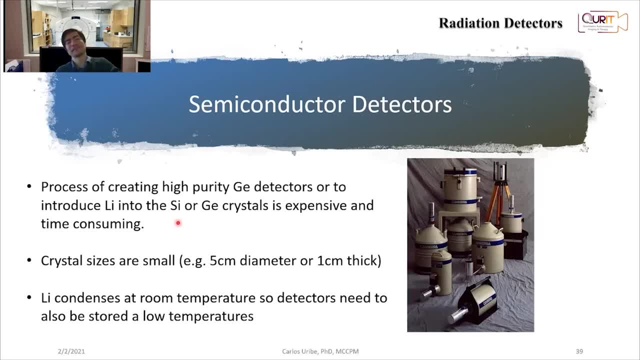 for those crystals to compensate for the electron traps is very expensive, though, and it's very time consuming Crystal sizes- we cannot make them very big. They're small- typically five centimeter diameter would be typical for a germanium detector or a silicon detector- will probably won't be able. 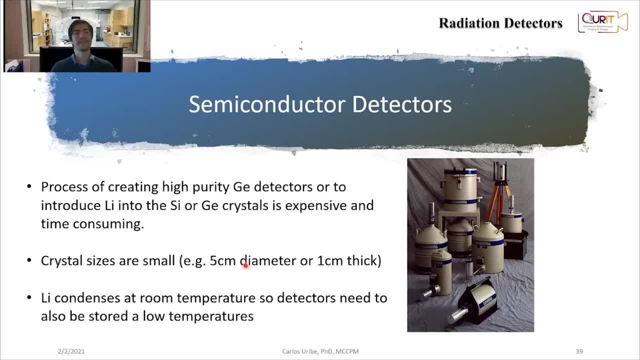 to be made more than one centimeter thick. And the other thing is lithium, and that's why I was saying about lithium condenses at room temperature. So yeah, that's the reason why those germanium doped with lithium detectors need to be stored. 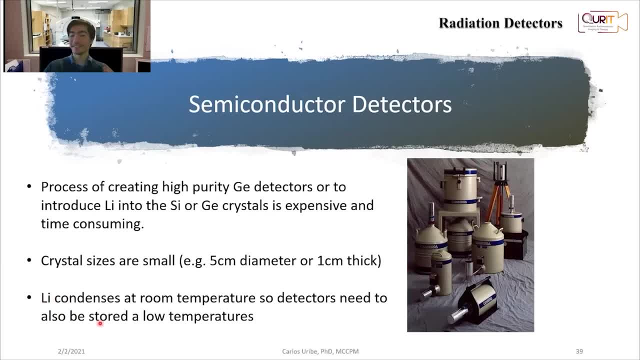 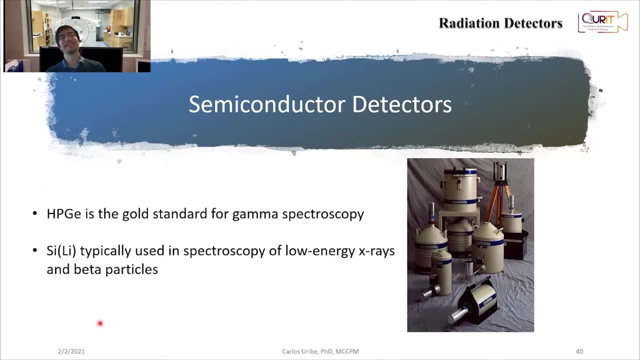 at very, very low temperatures, because otherwise this lithium just condenses, and it will just damage your detectors. High purity germanium, though, is what's become the gold standard for gamma spectroscopy. So why is gamma spectroscopy? Gamma spectroscopy is when we have a sample. 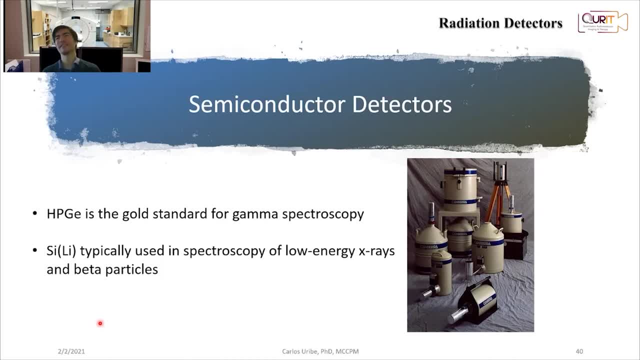 and we want to see why are all the energy emissions, for all the energies of all those, all those gammas that are being emitted by a sample, So you can do a graph of different energies and how many photons of each energy you have, because of the high resolution of germanium. 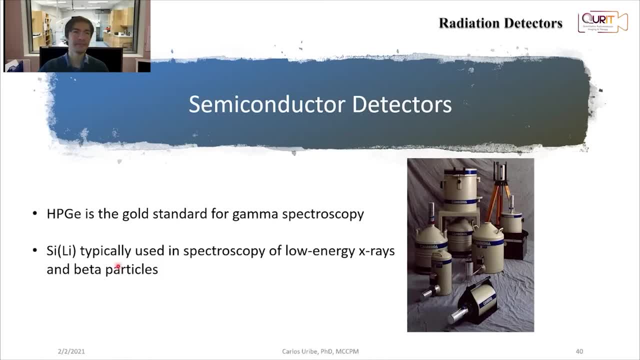 is very, very used in these applications And silicon is typically using spectroscopy of low energy x-rays and beta particles- Again similar when we want to measure the energies of a sample of different betas and x-rays with low energies- CCT detectors, as we saw. 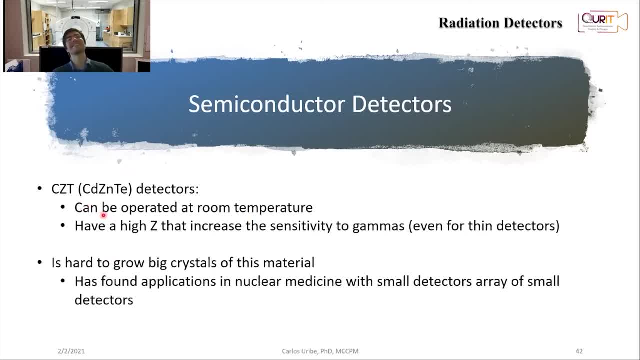 can be operated at room temperatures And because they have such a high Z, this increases the sensitivity to gammas, even if they are thin detectors. Even if they are thin detectors, we can still measure a lot of the gammas. However, again as I said before, 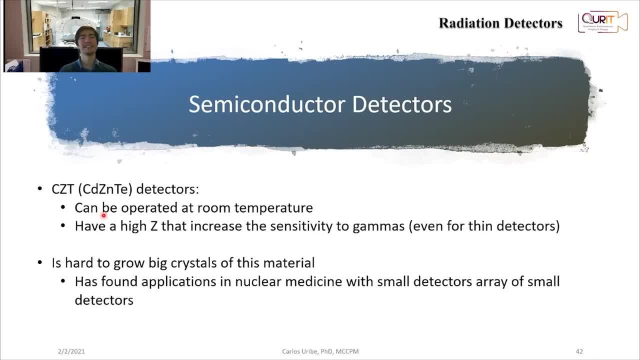 it's very hard to grow big crystals of this material. So it has found applications in nuclear medicine, but only when we can use small detectors or an array of small detectors. Now they're still expensive. Even making these array of small detectors becomes very expensive. 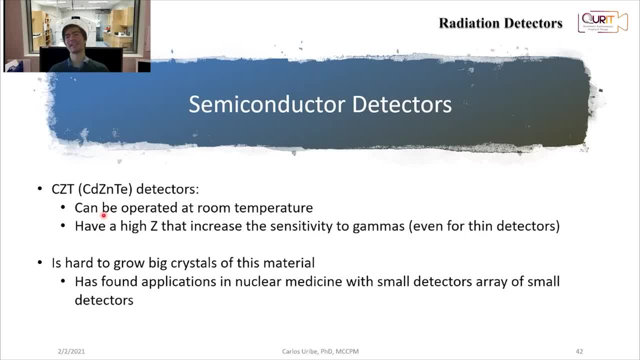 So we're starting to make it into the clinic. There has been some cameras, typically used to image the heart that are becoming more and more popular, but I can think that as technology keeps advancing, hopefully they get more and more popular, And one of the reasons 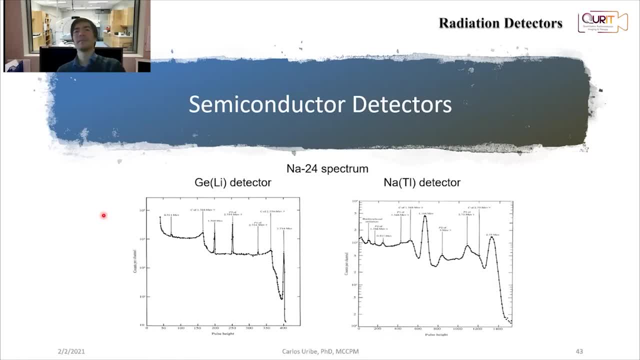 and I'm gonna show this more in detail. Sorry, But if you compare, for example, a solid state detector, like what we see on the left, and a sodium iodine detector, which we see on the right, which is a scintillator, 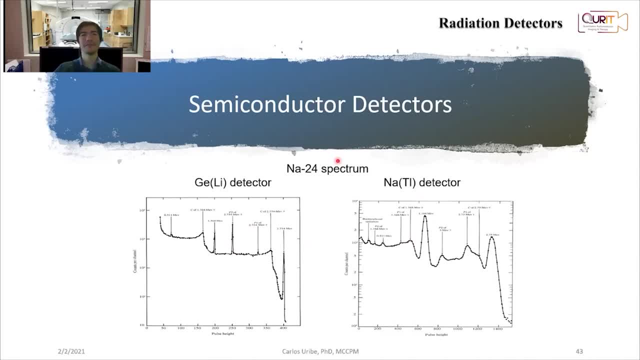 and you wanna measure energies of photons. in this case it will be the sodium 24 spectrum. Look at, for example, these energy: 2.75 MeV. The sodium detector gives you a very, very wide peak compared to the solid state detector. 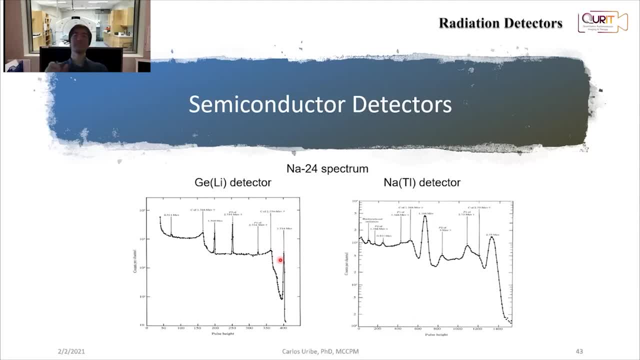 So yeah, so semiconductor detectors are very good at narrowing. basically, this is something that we call energy resolution, and we're gonna get into more details about what energy resolution is. but is that energy resolution in this particular case that makes it so good for gamma spectroscopy? 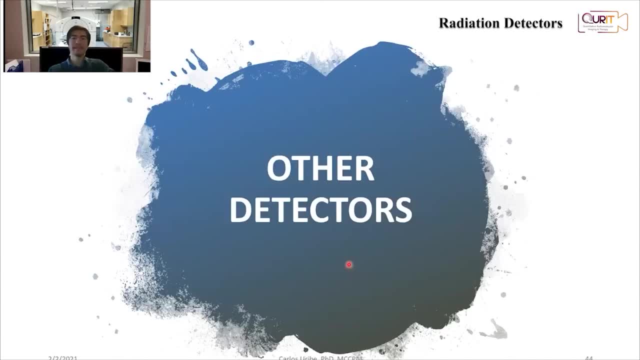 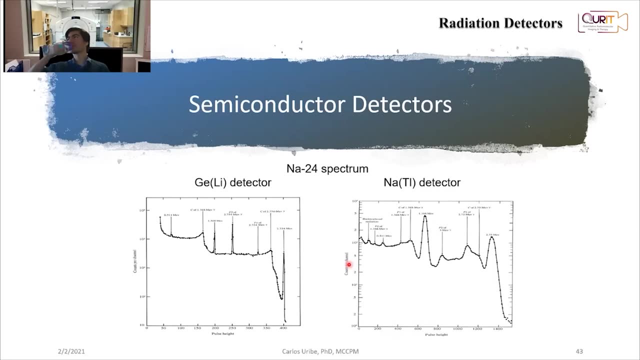 compared to other types of detectors, If I may, if I may, just add a comment: Yeah, and discussions, lectures, we will see, especially when we talk about some new exciting, state-of-the-art SPECT imaging devices, that there's a lot of action happening on CZT or CZT. So you know. 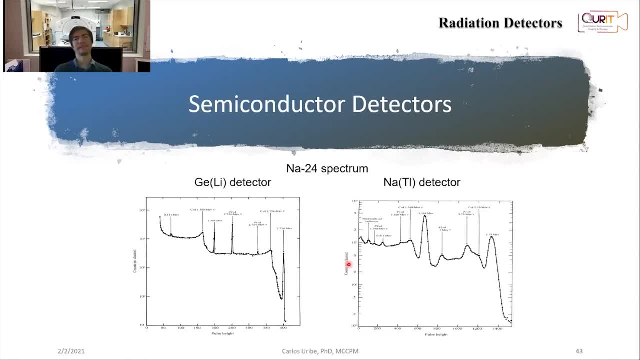 stay tuned because we're going to talk more about some specific examples of that, But you're going to keep hearing about this, even though we're going to talk about scintillation detectors, which have been the primary sort of approach to detection of gamma rays, In detail. we're going 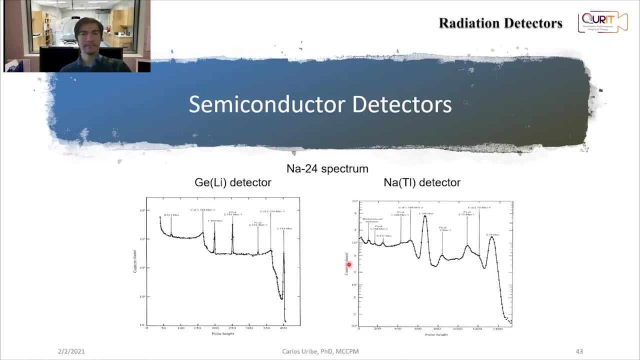 to talk about those. But again, semiconductor detectors are definitely starting to appear in your applications. Maybe I just realized, but you can think that how is that these detectors look? So you would have something like your solid state material here and then you have like a 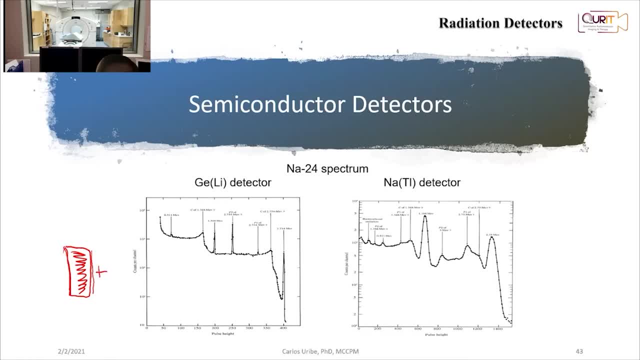 nail. So you have one electrode that you connect to the positive side and one that you can connect to the negative side. So when ionizing radiation comes into these crystals, that's when they create negative charges moving to the right and positive charges moving to the right to the left. 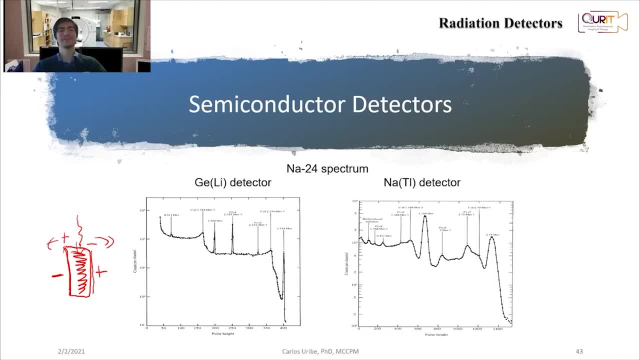 So we measure that current and that's how we're able to know depending on the pulses that we get. we know the different energies. But it's similar to a gas field detector, It's just that this instead of it's just in between the electrodes. instead of having a gas, now you have. 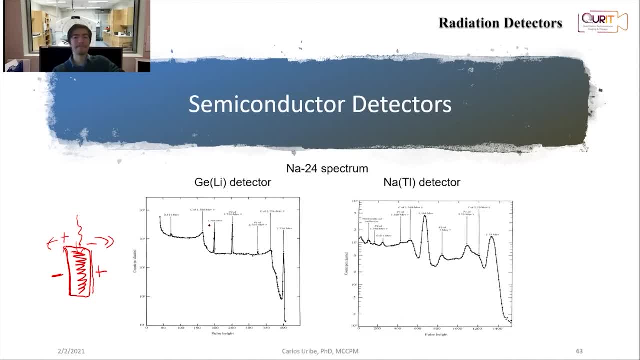 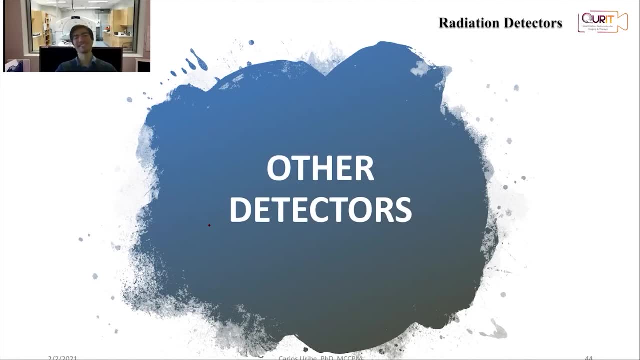 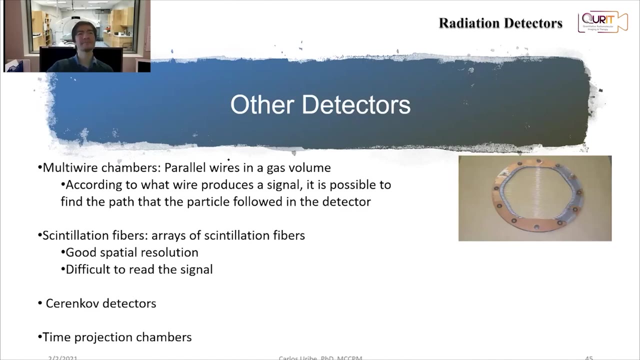 this solid state material. Now other types of detectors, and not necessarily using nuclear medicine, but it's just detectors that are used to measure different types of radiation. There's something called multi-wire chambers, So they're parallel wires in a gas volume. 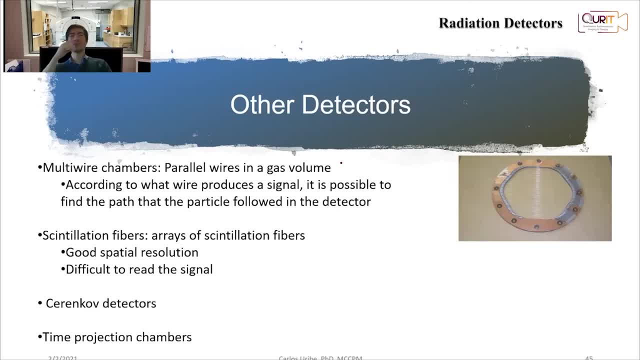 and these are typically used because according to which wire produces a signal, So you have a gas, but then it detects exactly in which of those wires, something like, as you look in the right, Depending on which wire receives the signal, then 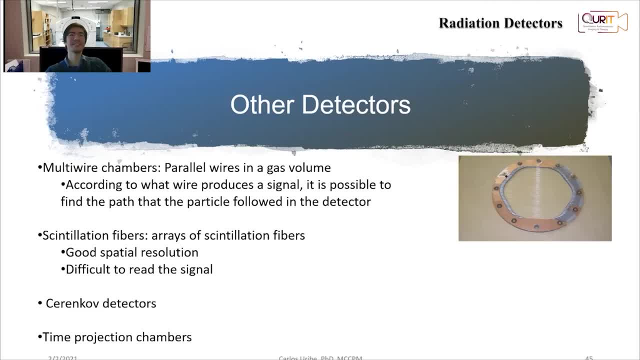 it's possible to track the trajectory that a particle is following inside that detector. There's also scintillation fibers, which are arrays of scintillators that they give you a good spatial resolution, but it's really hard to read the signal. 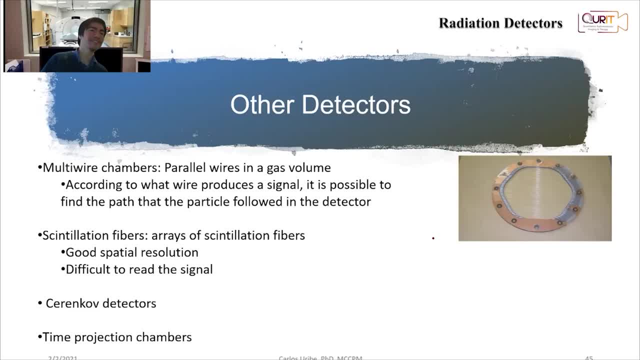 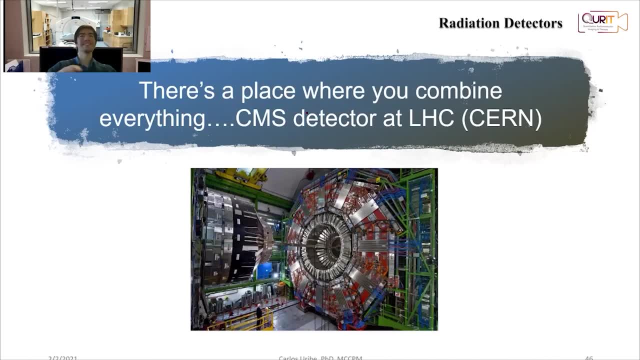 There are also detectors that are used to measure. for example, if you have a particle that has a magnetic field, you can use these detectors to measure Cherenkov radiation. There are some other detectors called time projection chambers and a place where you can combine everything and all. 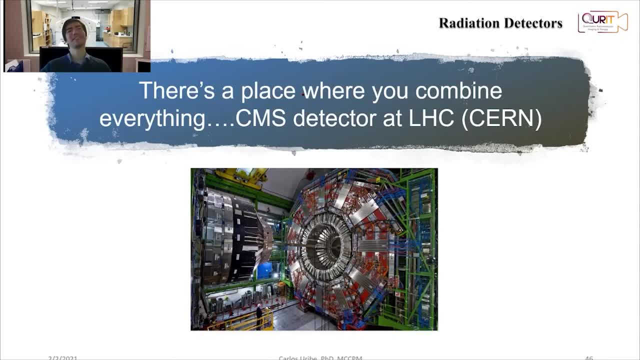 the types of detectors that I guess has been out. there is, for example, at CERN, at the Hydron Collider, where people are just working on detecting all types of particles of charged, non-charged and trying to look into understanding fundamental questions of you know.